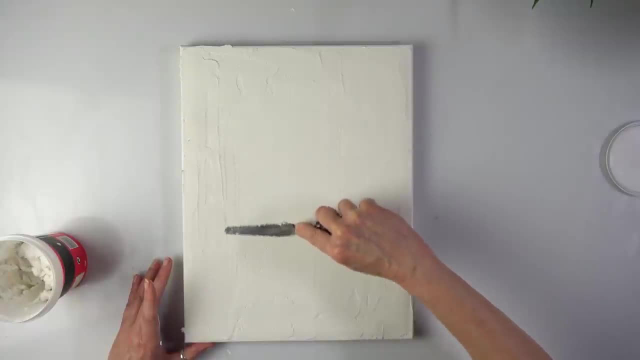 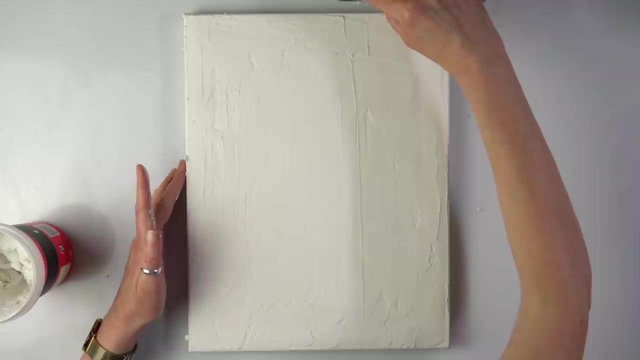 As you can see, I'm trying to make the mid part really smooth. Smooth and even because that's the section for the bluebells, The thickest are the corners in this case. But of course you apply it the way you like it. It's going to be heavier, of course, if you apply a lot. The main attraction today. 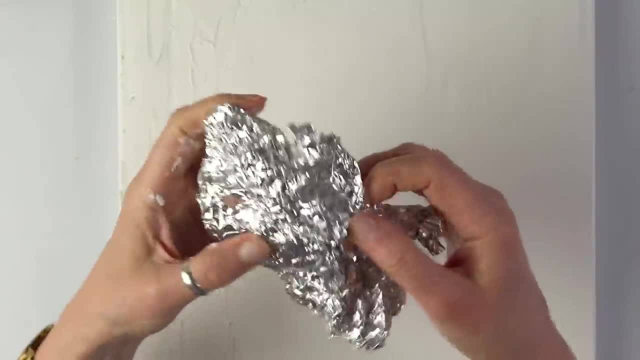 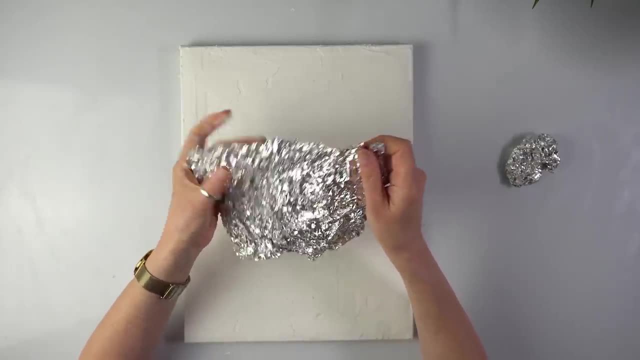 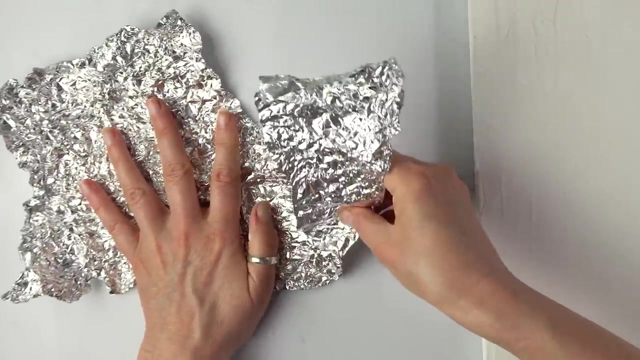 is going to be this: I've crunched it up to create some texture, Or if you scrunch it up more, your patterns will be smaller. I'm just going to rip it, And when I rip it I don't want any, even shapes, Something like that. 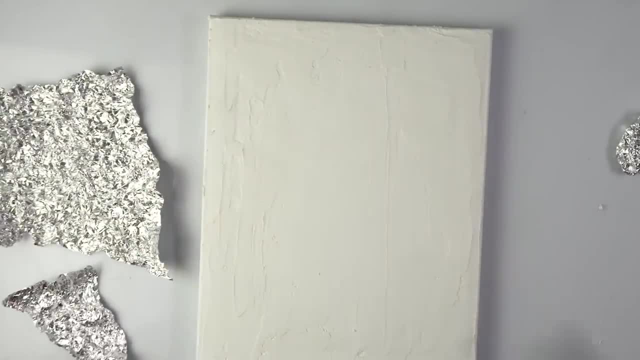 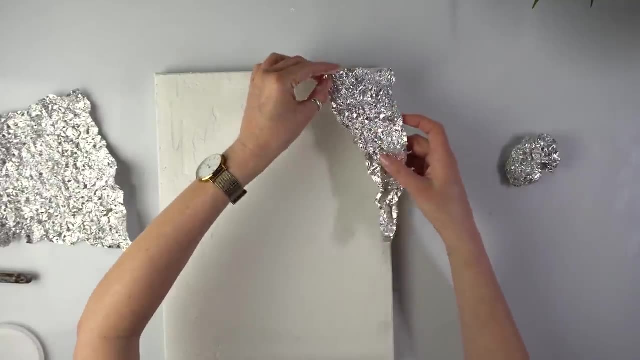 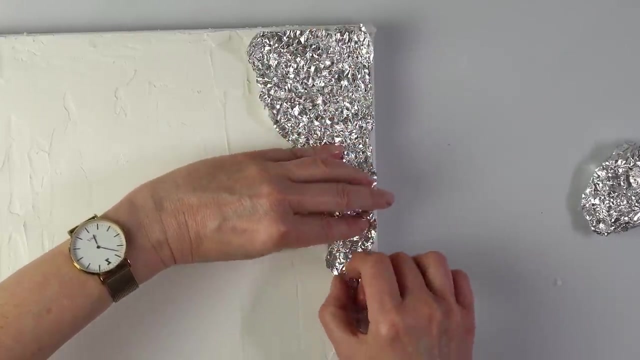 All right, I hope it's not too big. Let's see. Well, I haven't seen anybody using this with a filler, so I'm only hoping it's going to work. Why not? So if we attach it Somewhere like this, I'm so curious. This is the best part of not knowing what will happen. 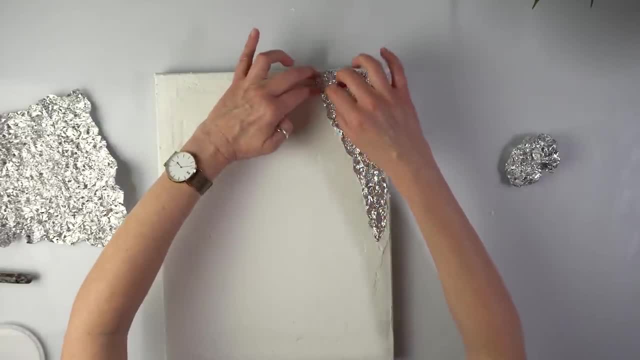 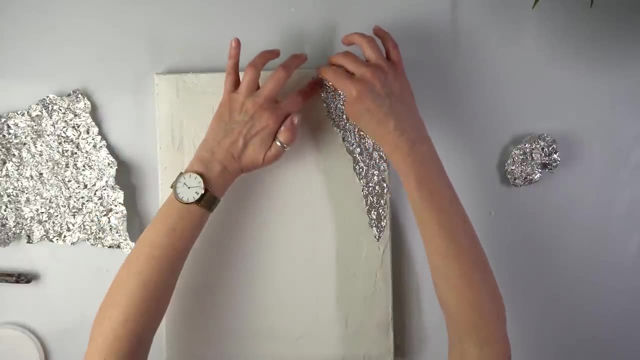 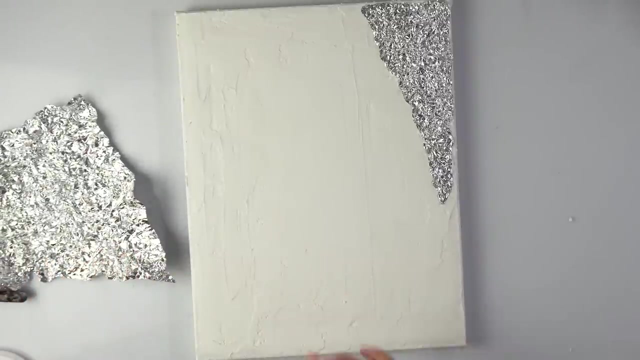 I'm hoping it's going to get stuck really well. What do you think? And thank you so much for always being so patient with me when I experiment and don't know what will happen Interesting? So I might use this lovely stringy bit as well, But let's just use this first A bit more. 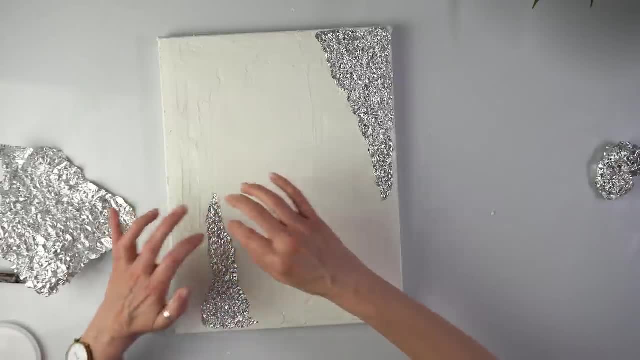 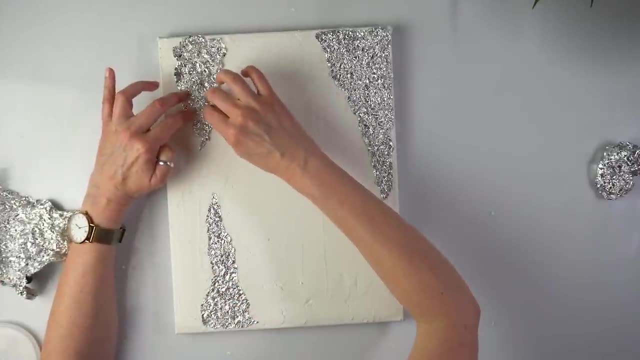 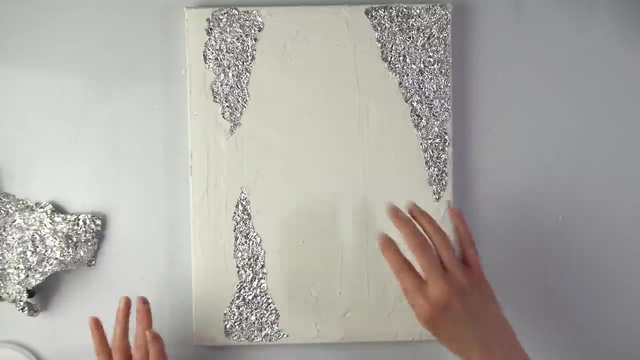 Random places. I definitely don't want it flat. I want it as scrunched up as possible. All right, Maybe here I'm going to scrunch this one up a bit more. Well, I haven't decided what to do once it's dry. Okay, Time for the stringy bit. 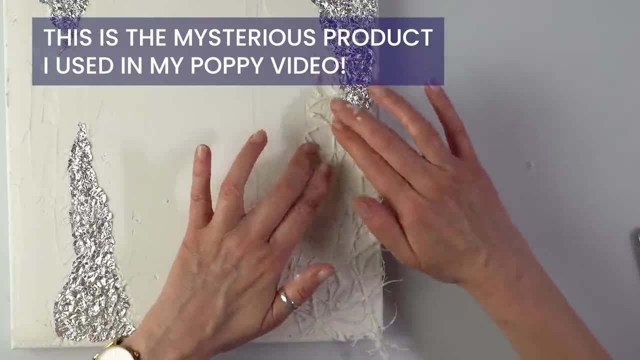 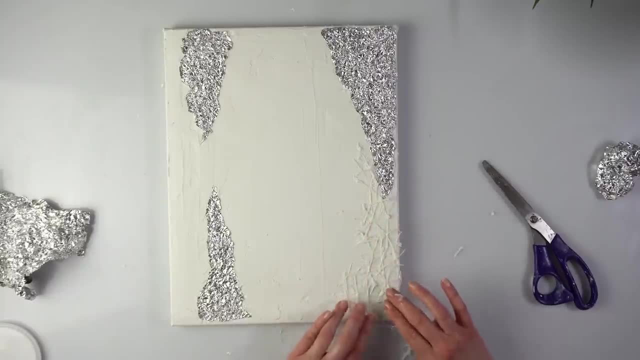 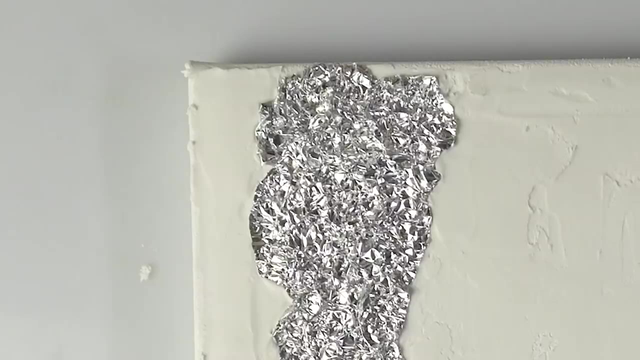 Pressing it down. Oh, there was not much here, So let's Whoops. You need a bit more filler for this type of texture. You can use string on its own, You know, scrunch up some string. I've got like little bits that can be attached as well. 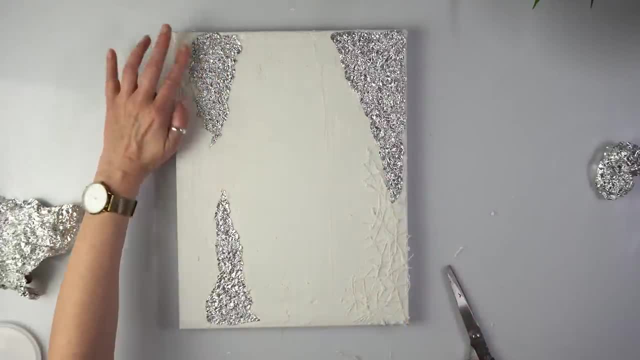 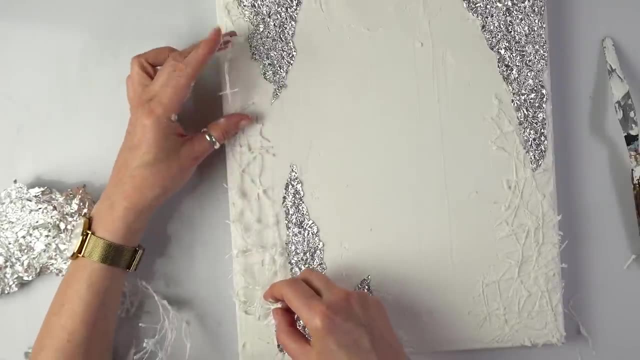 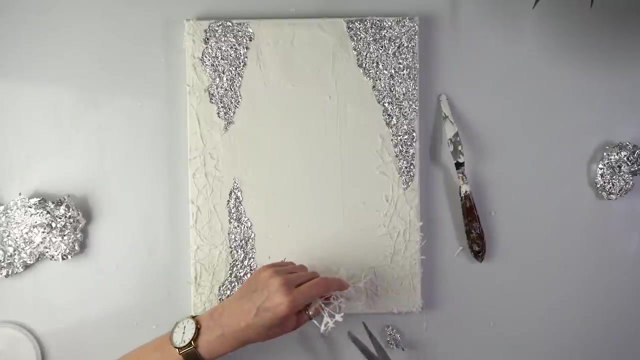 It will all be interesting And you can cut the edges later on, once it's dry or straight away. I want to put something in this corner, Actually maybe even that high, And just some at the very bottom. Don't want them overlapping because they won't stick well. 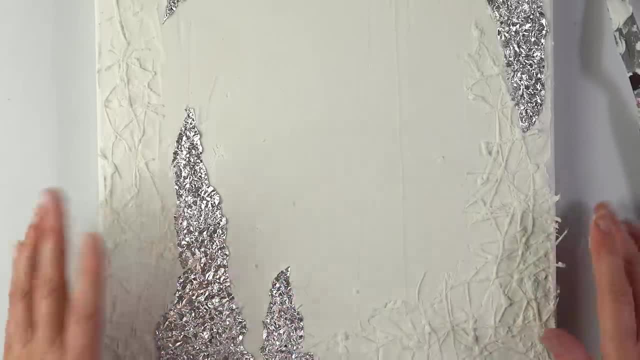 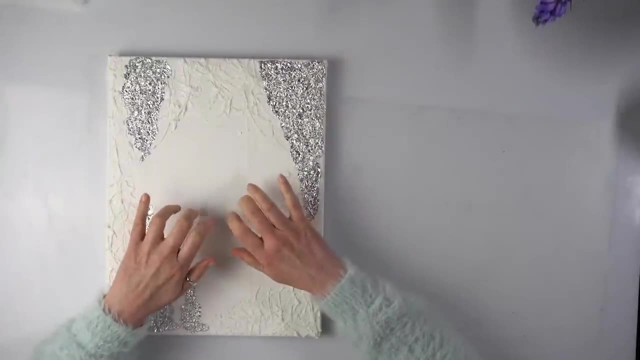 Oh, this is so much fun. Shouldn't take that long to get dry. All right, Just the top and we've got the midsection ready for our flowers. The background is almost dry And I'm going to prepare some leaves. I was going to use these. You can find them in the 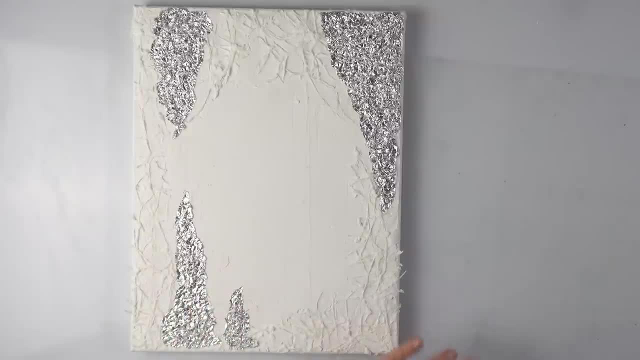 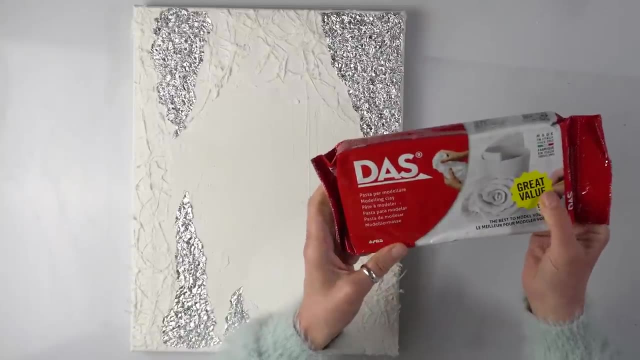 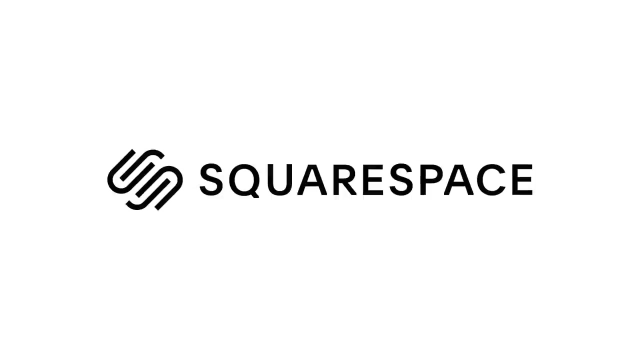 the same filler for the leaves. but then I looked around and I noticed that I have this and I've never used it before. It's not even open, so let's just see how this is going to behave. I'm sure it's going to be really nice. Now, before we continue, I would like to thank today's sponsor. 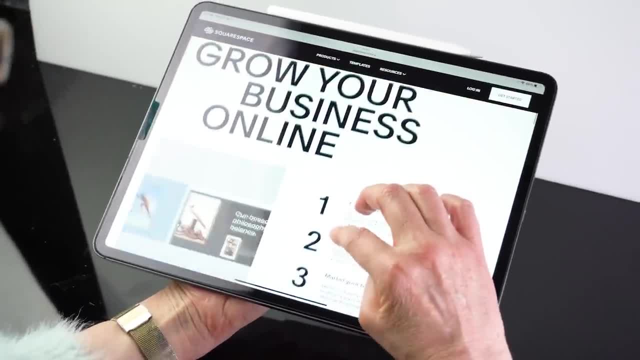 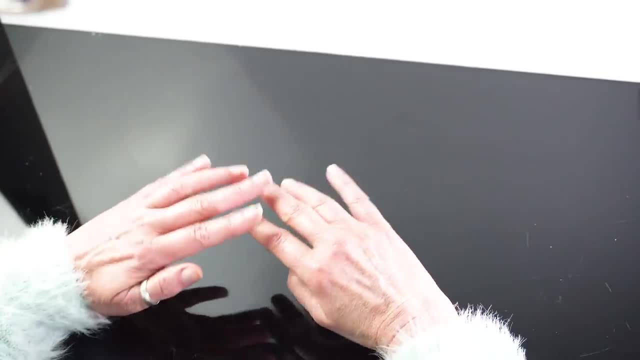 Squarespace. Squarespace is an easy to use online platform for creating websites. Have you always wanted a great, professional looking site for your business or hobby? Now you can make one yourself with no hassle. Choose from hundreds of stunning templates that you can easily customize and never. 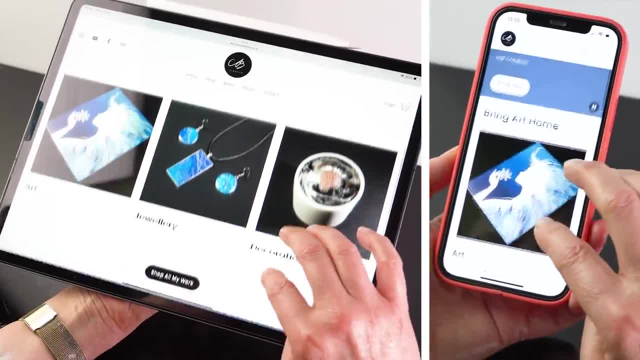 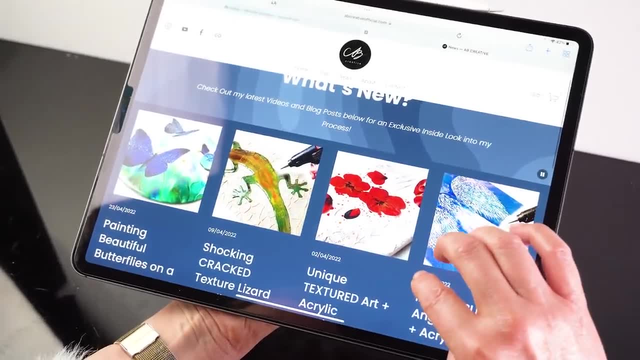 worry about updating anything. Squarespace automatically formats your site for both desktop and mobile. I even made my own website on Squarespace, and it's so easy to add new products and blog posts each week. Make any site you like how you like, by heading over to squarespacecom. 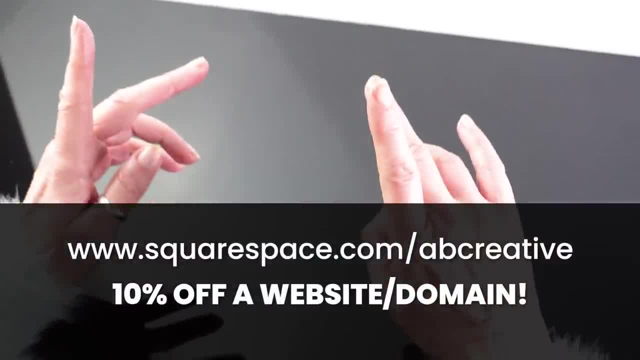 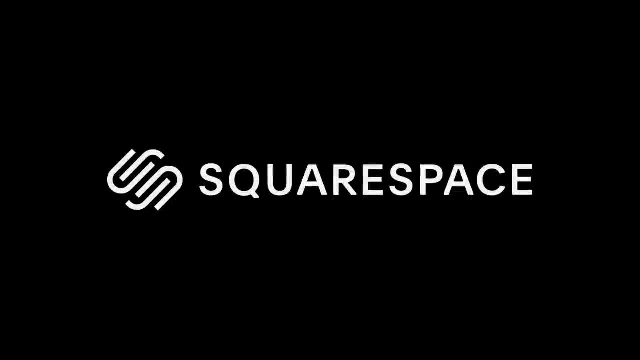 for a free trial and when you are ready to launch, go to squarespacecom. forward, slash ab creative to save 10% of your money. You can also purchase a website or domain and get your site up and running in no time. Thank you to. 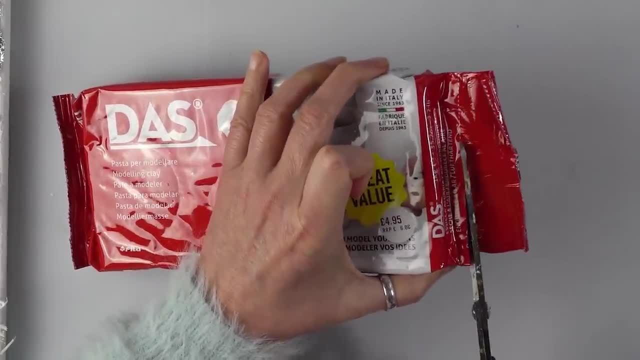 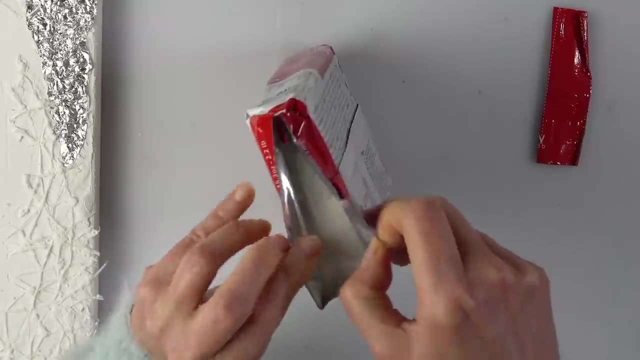 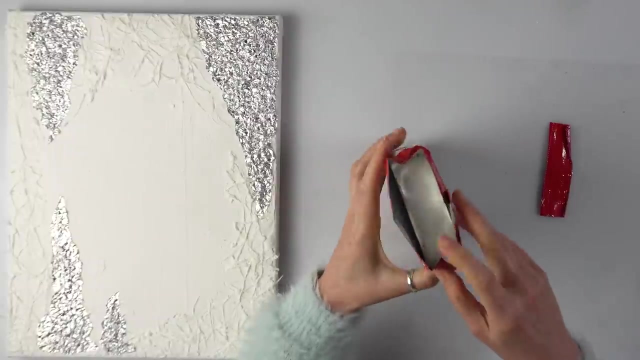 Squarespace for sponsoring this video. I think, since it's air drying, I'll have to have a airtight container to keep the rest of it. Oh look, it's white. For some reason I was thinking it's going to be brown. It's not. Oh, okay, I do work with normal clay, but not with air drying, with my. 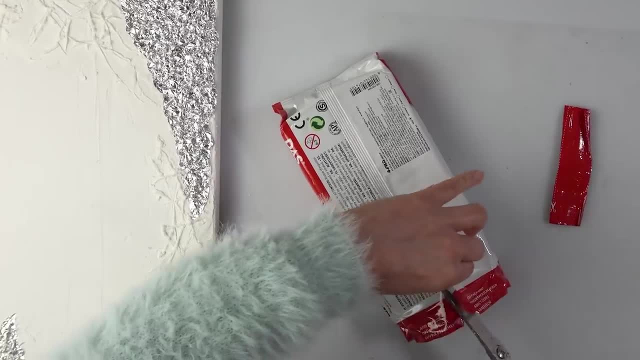 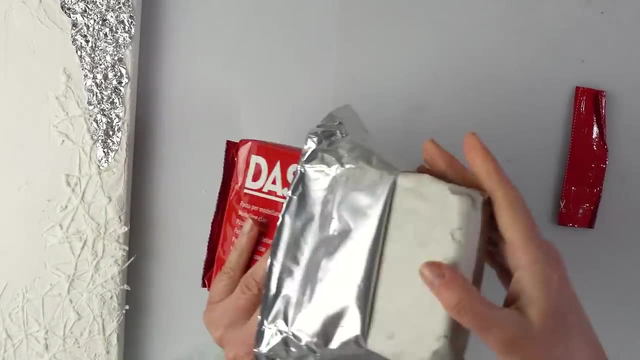 students. They're actually going to be doing a lot of work on it, So I'm going to do a little bit of painting. I'm going to be making food items tomorrow with my special needs group. It's a young adult, Absolutely lovely group. I've never used this. Oh, it's so soft. I'll be doing it on. 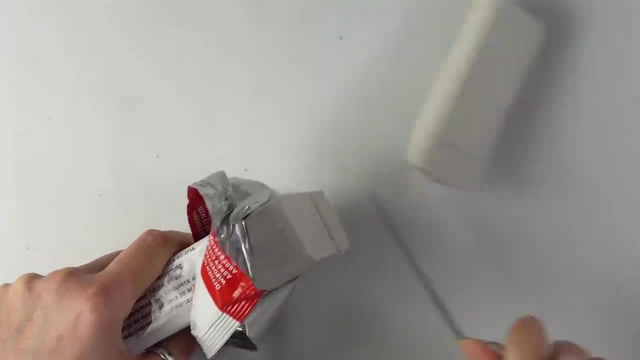 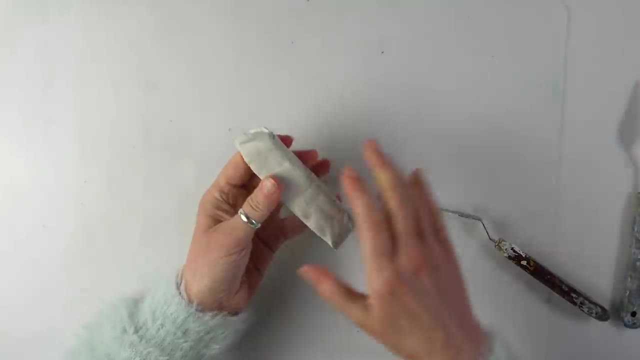 the silicone mat. It's a bit more sticky than the Fimo, So what do I want now? I'm going to shade the leaf and I'm going to press the actual leaf that I've collected. That will be the easiest thing to do. Let me split it. 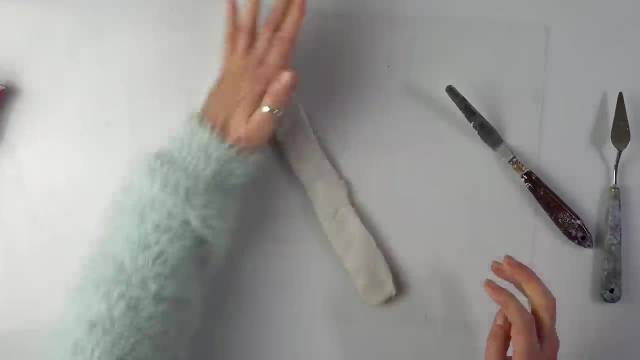 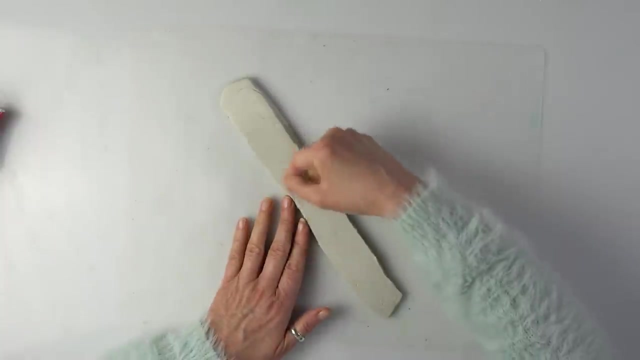 I want it long. Very easy, Super easy to mold. See if I can peel it off? Yeah, super easy. Okay, let's join in on this side. I want the leaf to be ever so slightly curved, So I'm pushing it in. 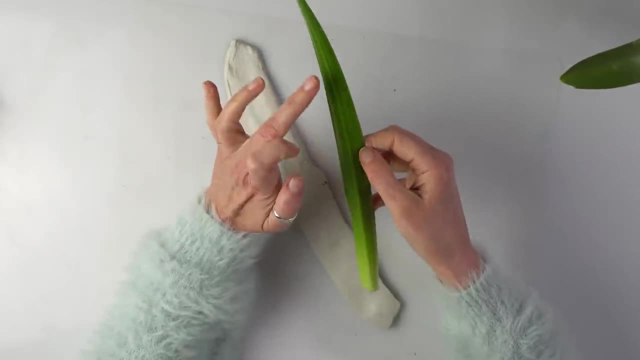 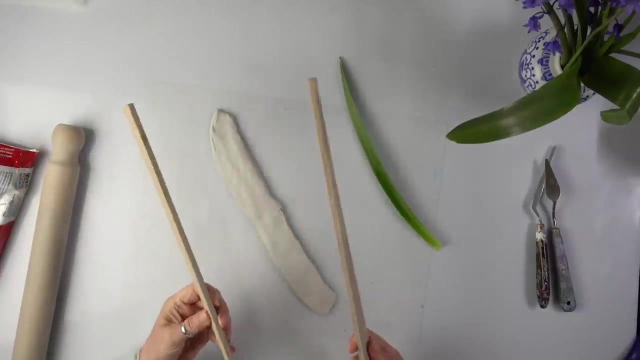 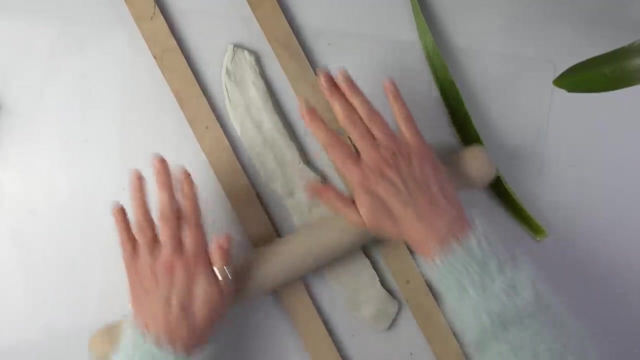 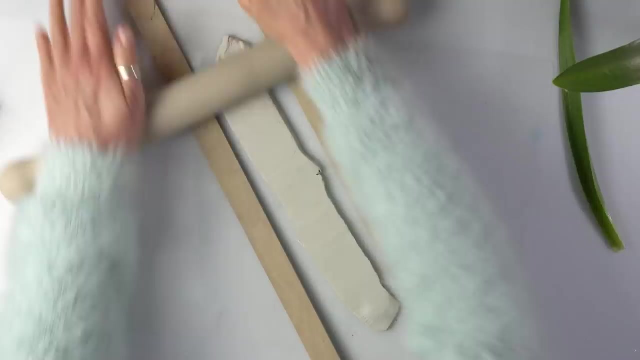 this direction. It's a very simple one. There's basically there'll be one line in the middle. It's so smooth When you roll clay. it's really, really important to have some wooden sticks just to keep your clay the same level, So it won't go any deeper than those two. It's going to be much. 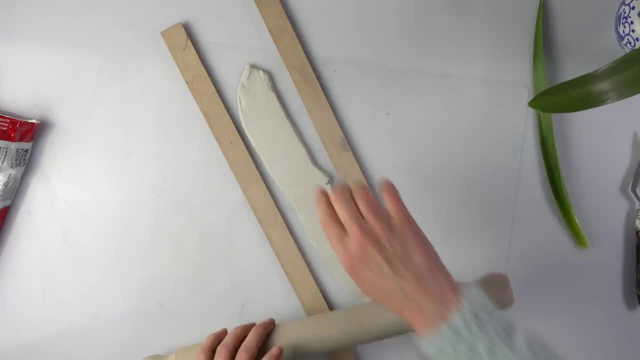 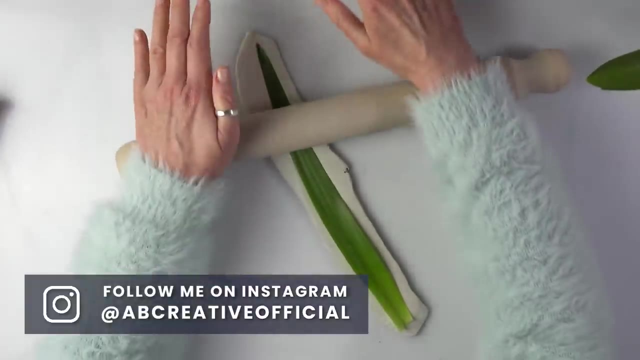 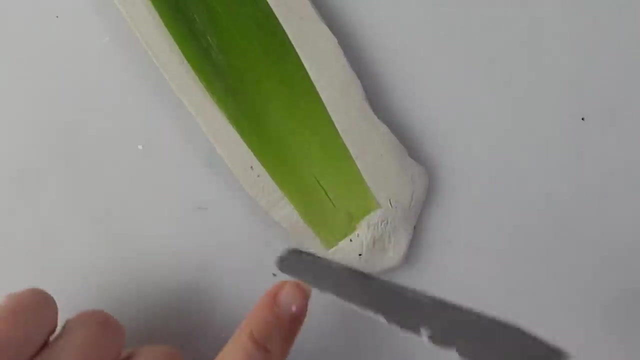 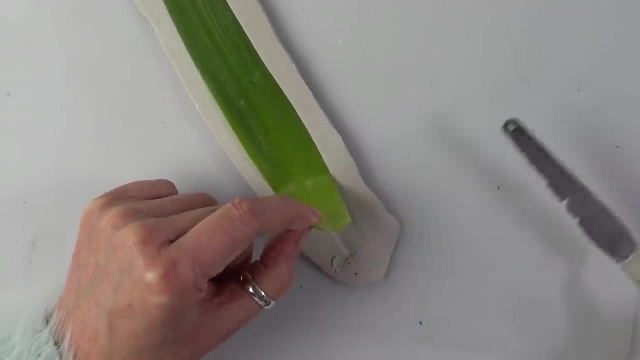 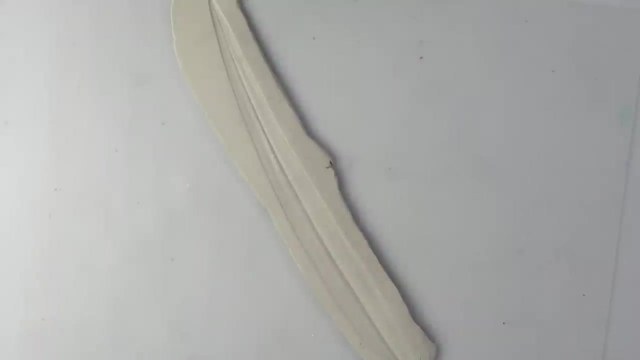 longer. Of course, it depends on your sticks how thick your clay will be. And now the imprint Some more And lift it up. Look at this beauty. That's what I want, And I'm cutting this out. Now you can use a normal knife. I'm just going to use this. 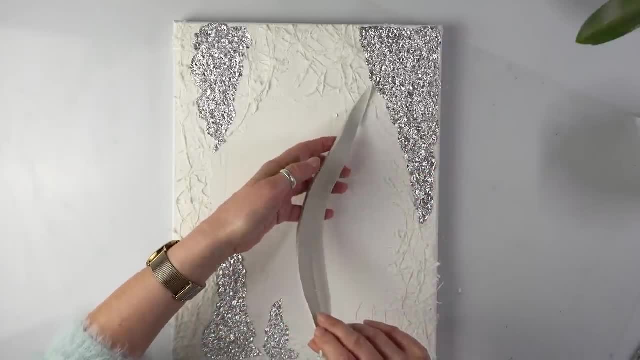 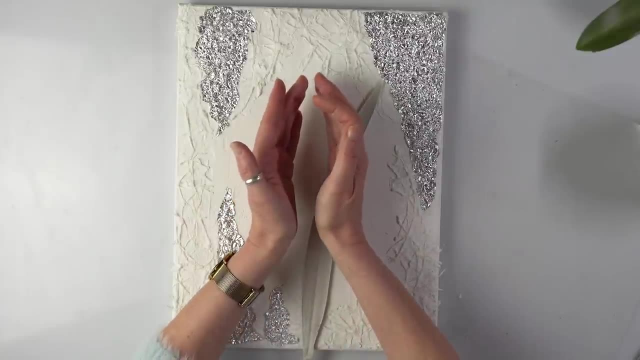 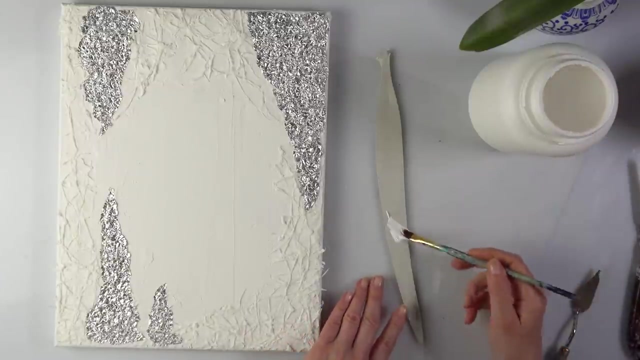 So this is ready. Now I'm deciding where to put it. All right, So I'm going to glue it. This is going to be- there's going to be a main flower. How about gluing this here? As I said, I did not use it before. I'm just hoping it's going to work And, as you've noticed, I'm actually 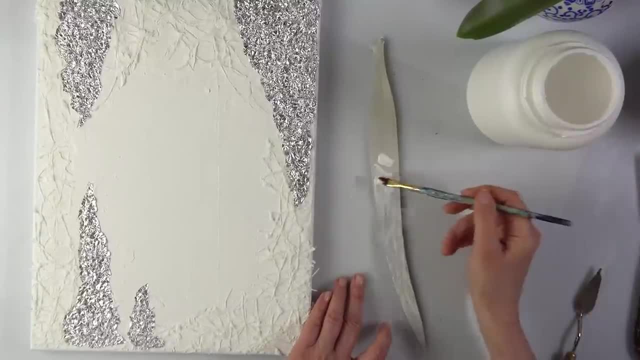 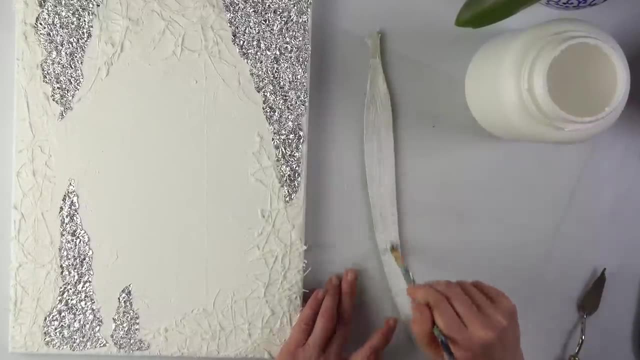 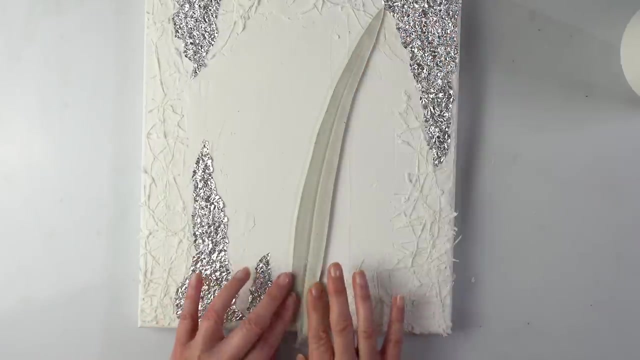 gluing it wet. There's nothing like experiments. you know, I'll probably need two or three more leaves And then I'm going to roll a stem for the flower. Just for now. It's so thick, So I'm pressing it down here, Making it flatter. 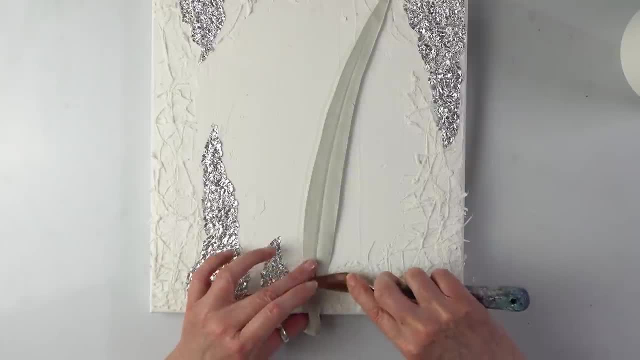 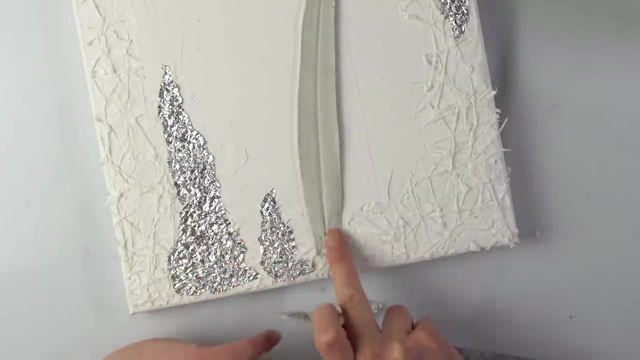 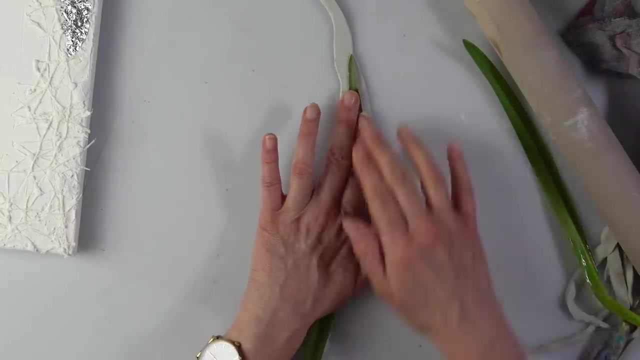 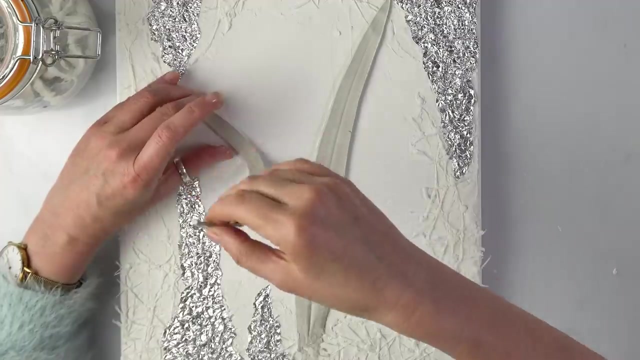 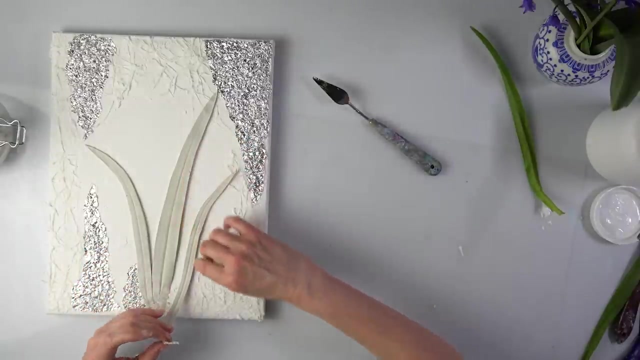 And then I'll remove this section completely, Just shave it off. I'm sure some of you work with drying clay So you can share your expertise with me. Send me some pictures, please, of your work. I'm going over my texture Just thinking where the flower will go. I have to really think now. 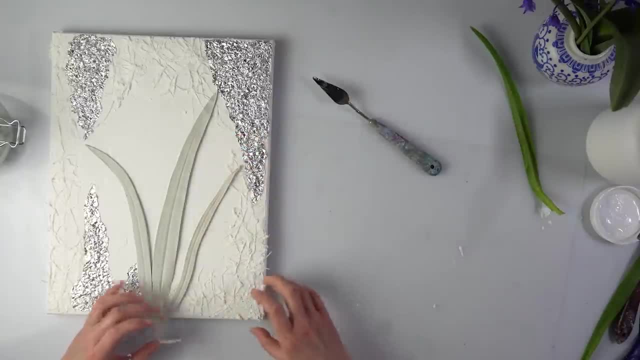 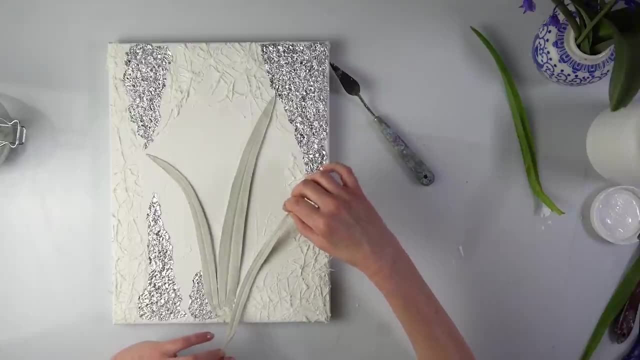 That's probably a good place for the flower. Therefore, the leaf will go lower. The last baby one. Now this one is so thin I wasn't sure I can pull it off, But I did want them thicker and thinner, Just to get the impression you know Some of them. I ended. 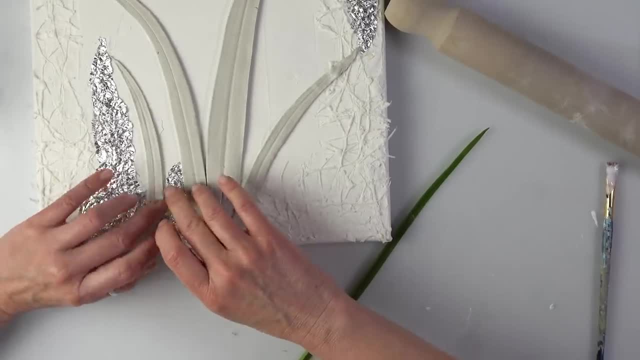 it further. Some of them I pulled it off. So I'm just going to pull it off And then I'm going to put it on the other side, And then I'm just going to pull it off, And then I'm going to pull it off. 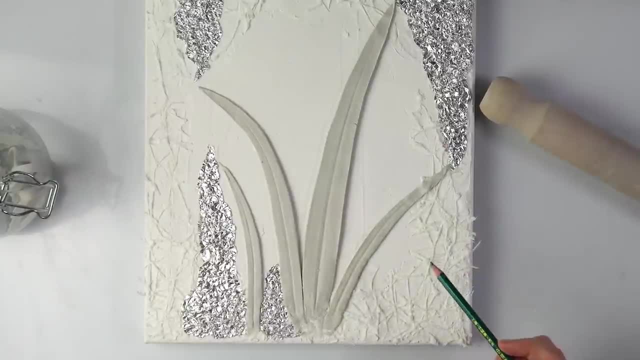 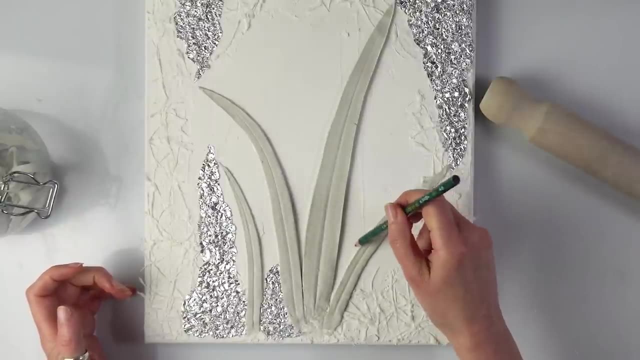 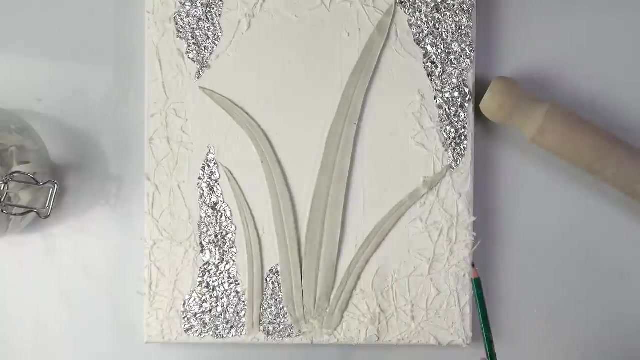 Closer to us. I'm going to sketch now how I want the flowers to be. I want somewhere here And it's going to be going over the stem Somewhere, Somewhere like this. Now the big one is, I think, is going to reach up to. 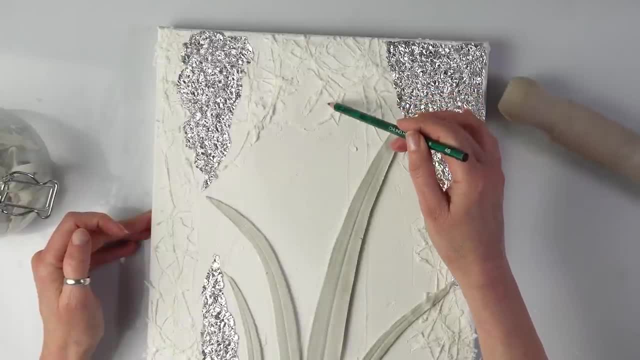 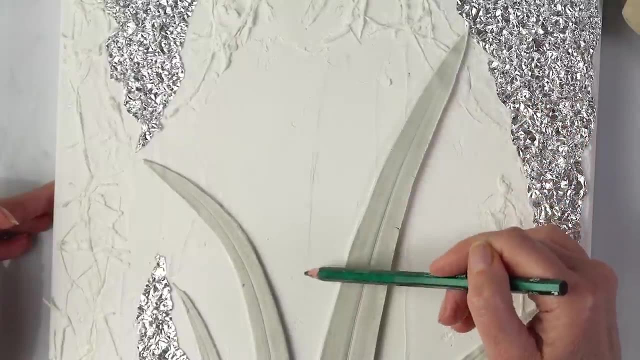 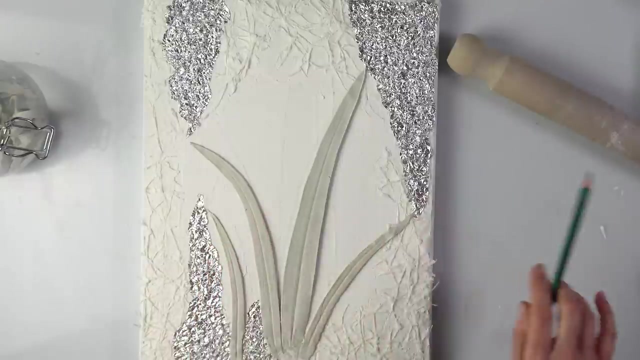 this section. So this is the highest point And it's going to go over the stem Somewhere here. You'll see I'll explain why I am not attaching the stems now. I am just going to make the indents. So I am taking again the real stems And I am going to 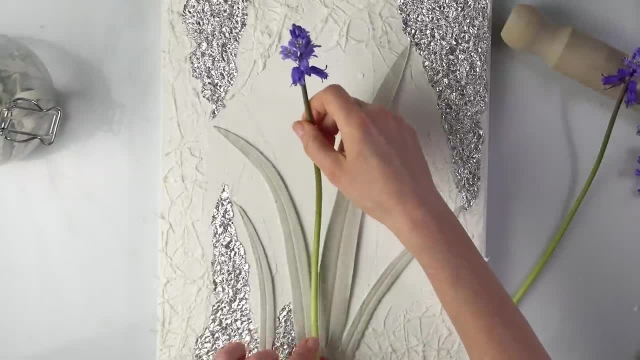 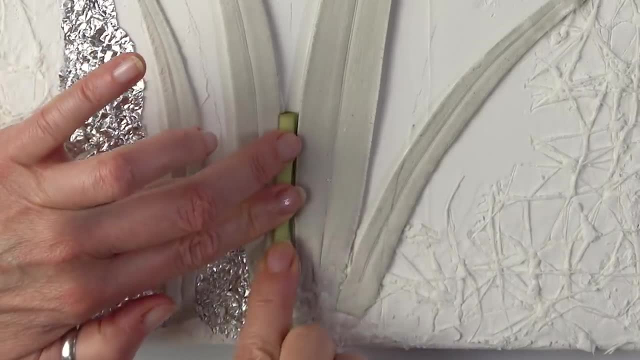 press them down. These are roughly same. So now I am making an imprint in my clay here for the stem here, So then it fits. So I am just going to make these, I am putting them down here, So then they would go above my stem. So then I am making the stents, Then I am going to press them down. These. 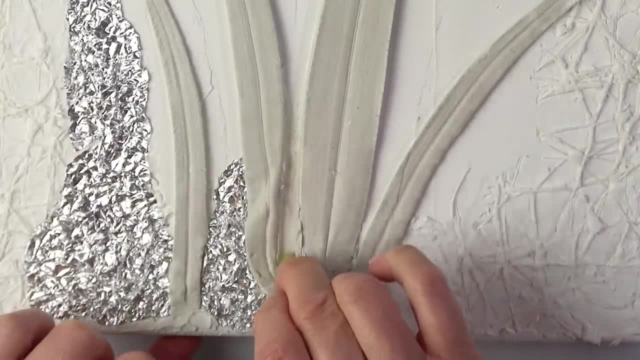 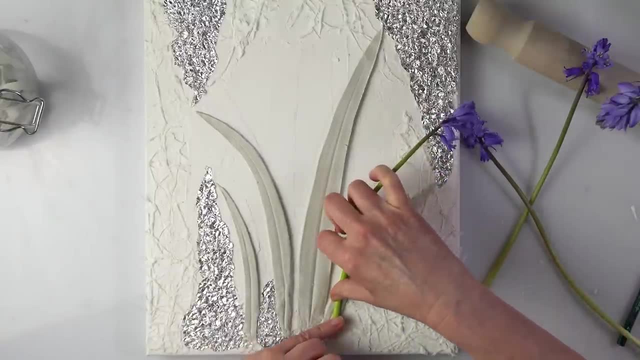 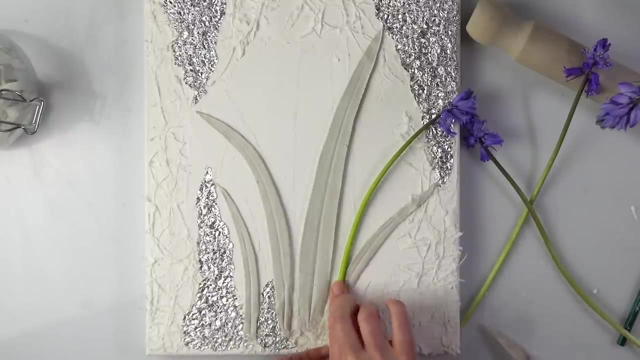 even thicker. So this is my place for the stem. There is one more that's going to be somewhere here, so I am only pressing it like this. You probably noticed that if I can use natural forms, I will too, you know, to get some special effect, and I 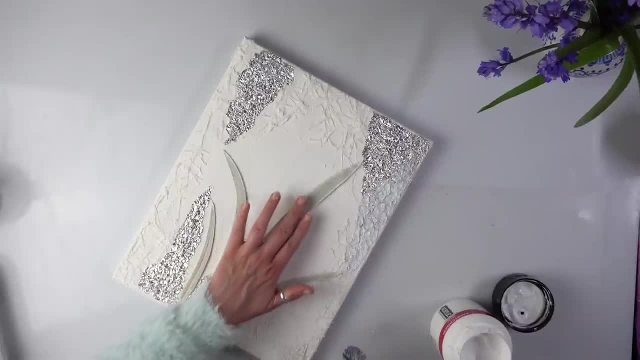 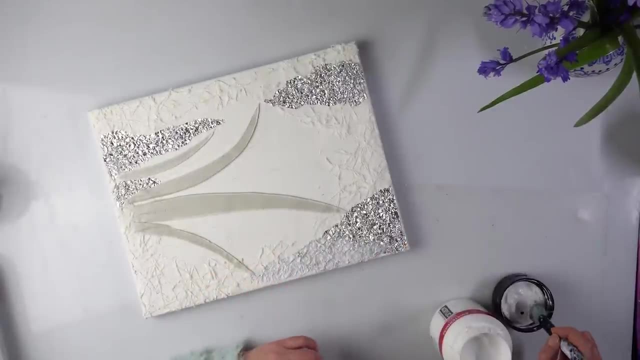 think that's going to work really well. While I'm waiting for the leaves to be dry, I've decided to just use my very soft brush- This is actually my makeup brush- it used to be- and I'm dabbing some white here before spreading any colour. 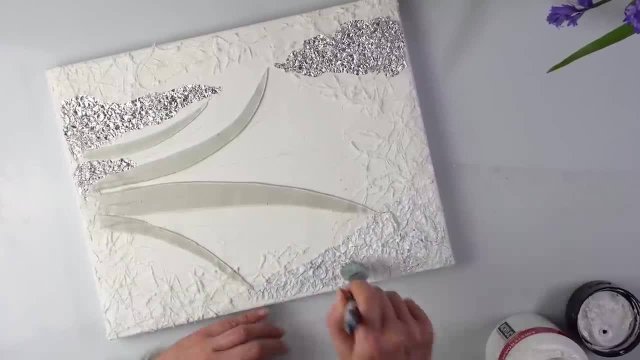 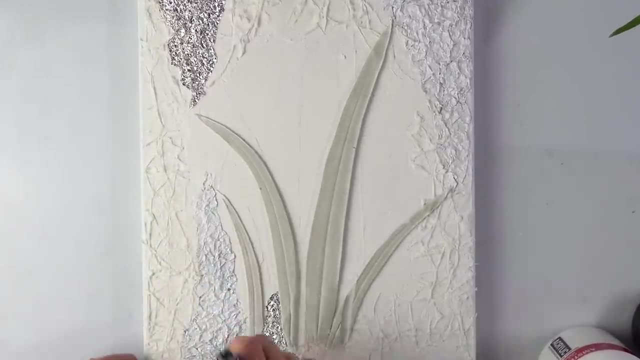 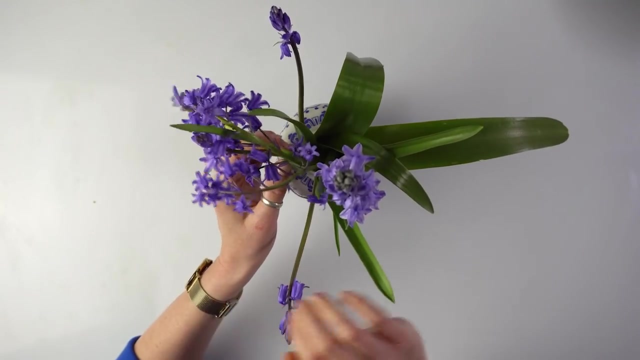 that I decide to use. I'm loving it so far. Another way you could cover everything is with spray paint. It'll be very effective. So I went for a walk today and these grow in woodland areas and sometimes they cover the whole floor of the forest and they are so amazing. So this is the inspiration. 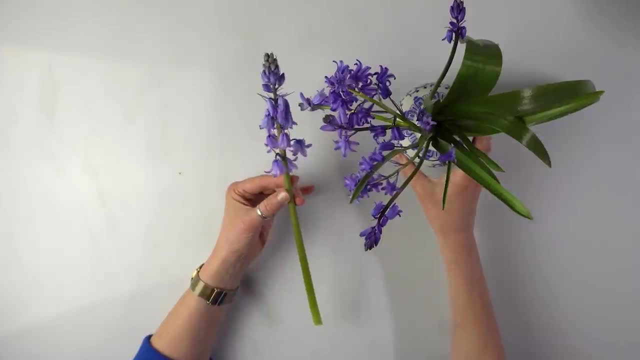 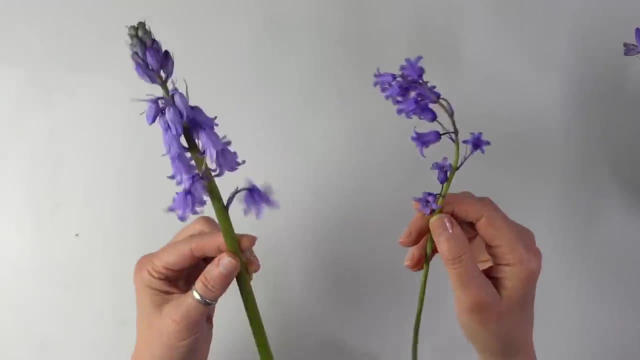 I found one really chunky and I was thinking I really want to make a piece with bluebells. They are the same family as hyacinths, aren't they? That one was growing in the sun and these were under the trees. I was thinking maybe I could make. 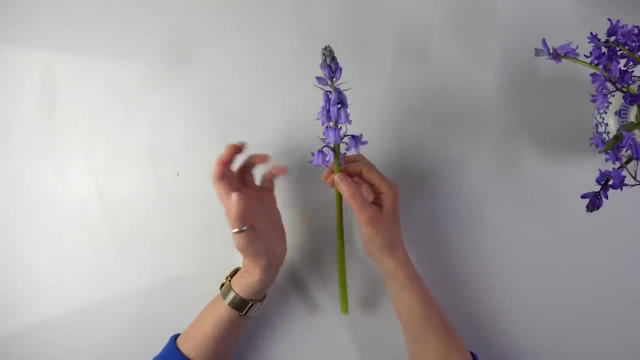 a mould. I was really, really thinking and I thought maybe I will use the filler, and the same ones as I use with the poppies and the peace lilies. I don't think the filler would make the case for a piece, because it's so easy to make it. 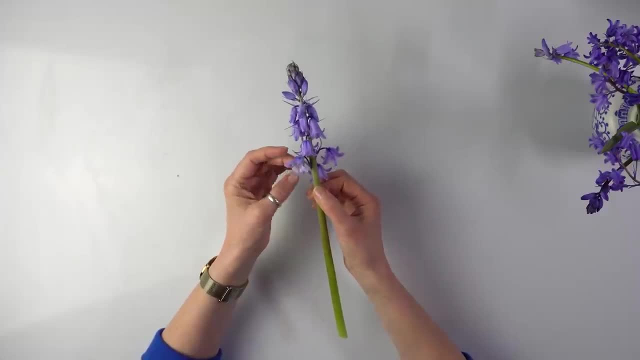 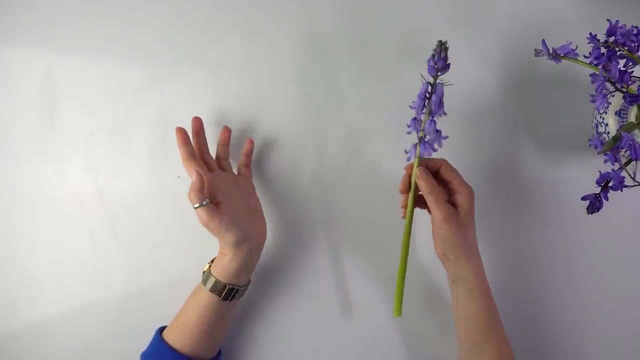 with my hands. It's really hard to make a mould. that's as difficult to do with the make me actually make those really delicate endings on the flowers. look how pretty they are. so in the end I've decided to check if I can make it from Fimo. I've got some left over. 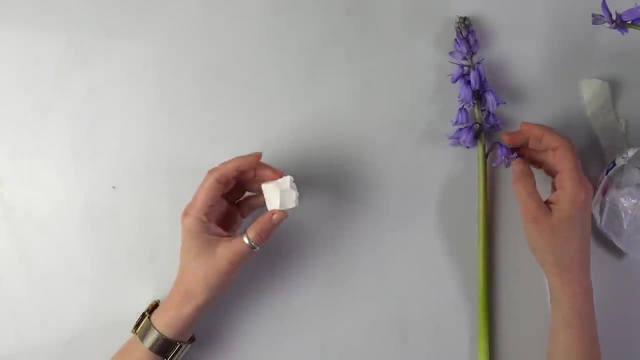 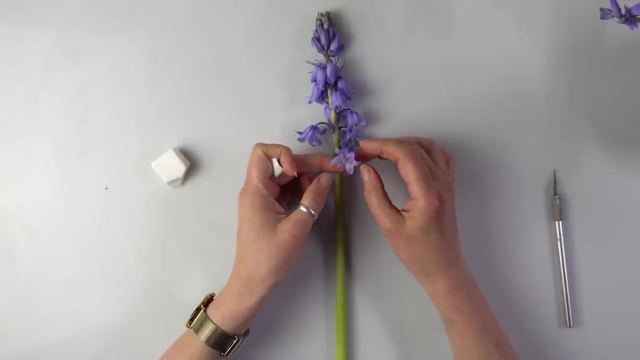 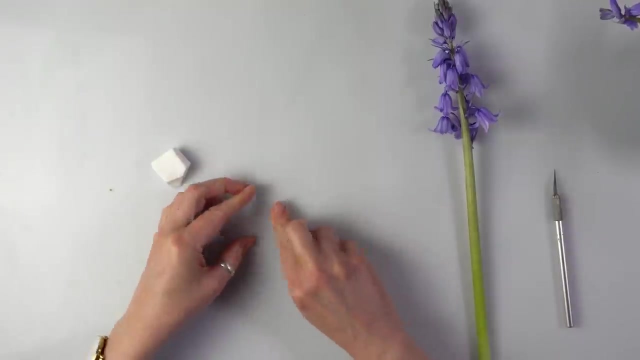 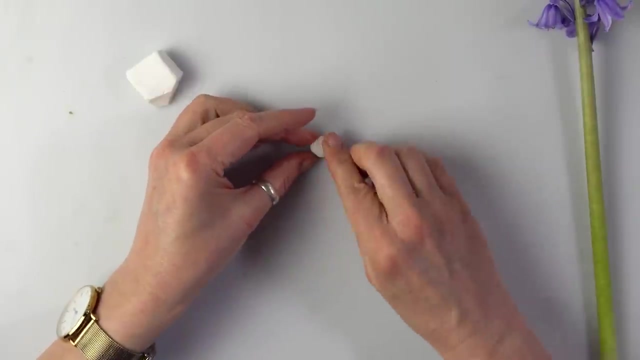 let's just test it first. how should I make it? I welcome you to my testing ground. you know I haven't done it before, so it's going to be fun for me and hopefully for you as well. so six petals- let me just think I'll roll a ball and I have to be chunky here and the petals are quite slim. so if I 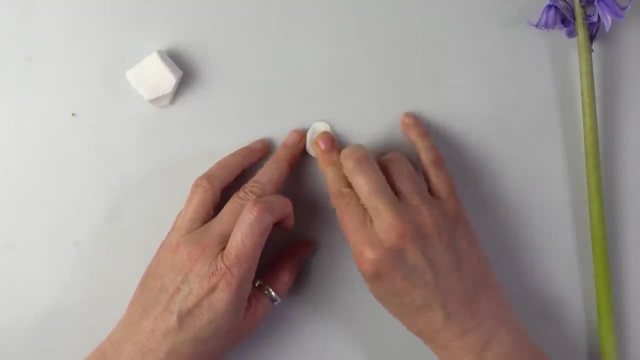 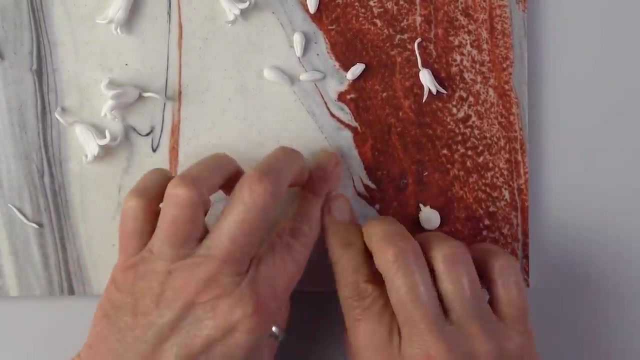 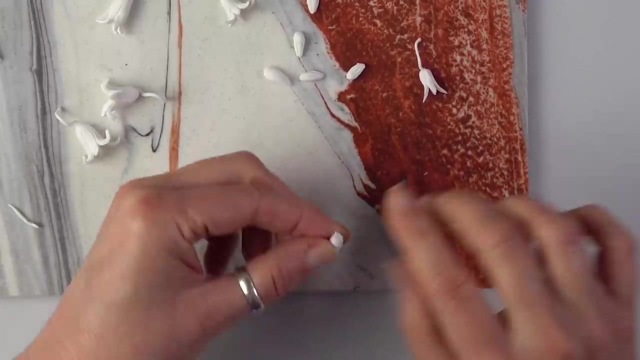 press it just like this. okay, so I actually took a little time off camera to figure out how to make the bluebells, so let me show you how. I've also noticed that working on the tile is so much easier. so you basically roll quickly here and you can lift it up. show you. 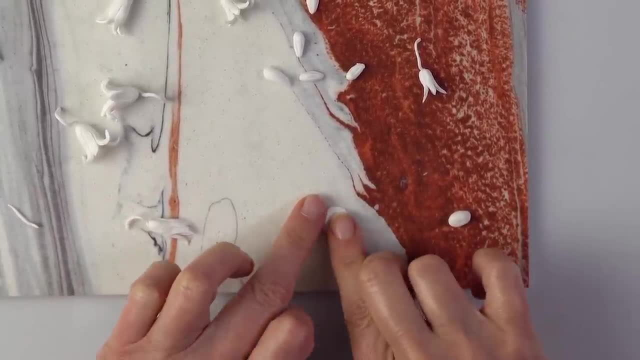 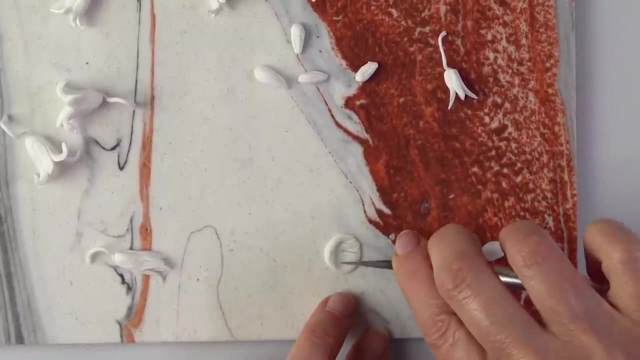 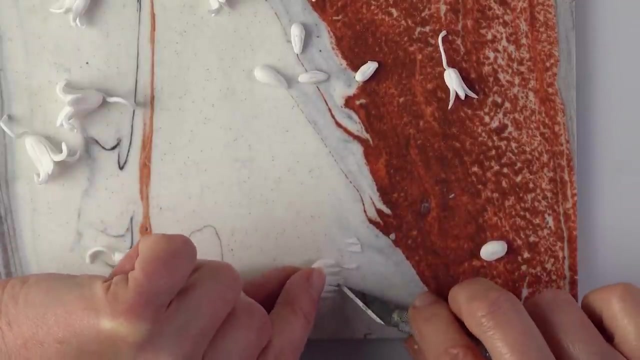 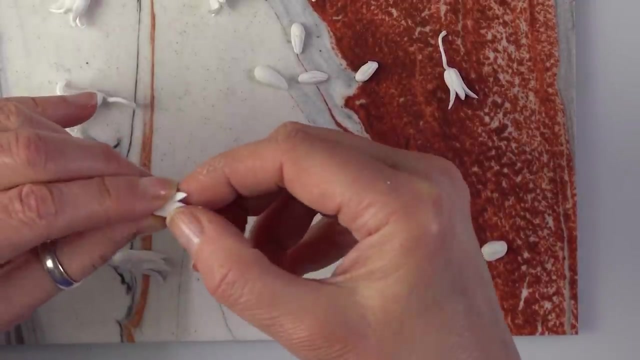 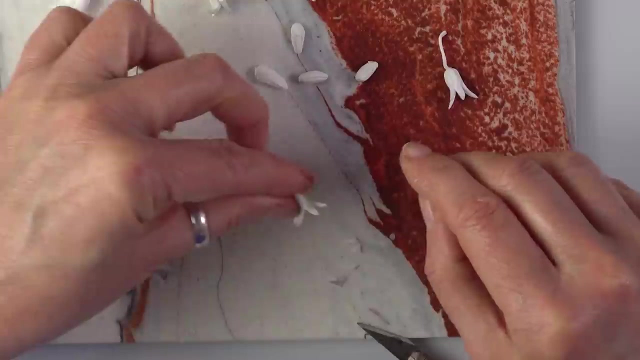 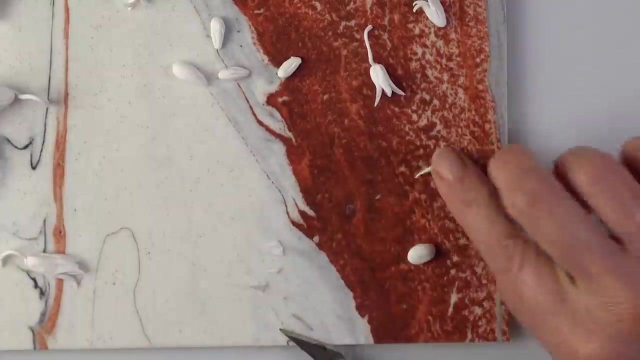 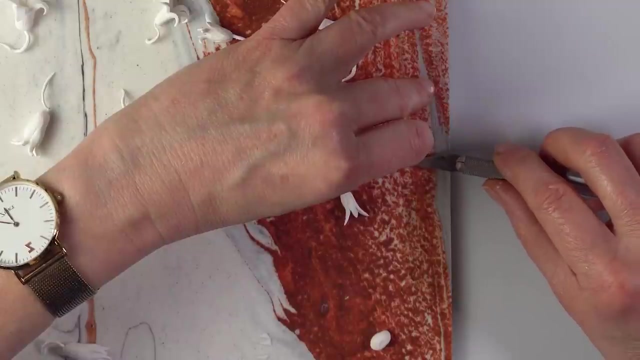 okay, so I flatten my section here, cut my petals and once I lift it up, all the bits stay, stay on the tile. so that was a nice bonus. just put a very small one together and put the spin, and now I'm going to put them in the oven with the tile, I'm not going to lift them. up. I'm just going to carry them and I will find more: 110 degrees for roughly 20 minutes. that's what they say. I don't think we need any more, do we? these are back from the oven and I must say the tile was the perfect thing to bake them on. oh my goodness, they're like a rock. 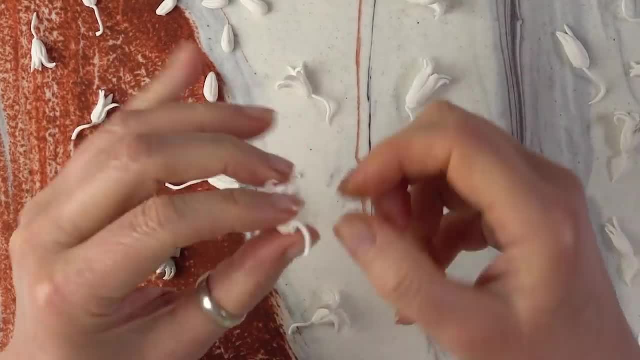 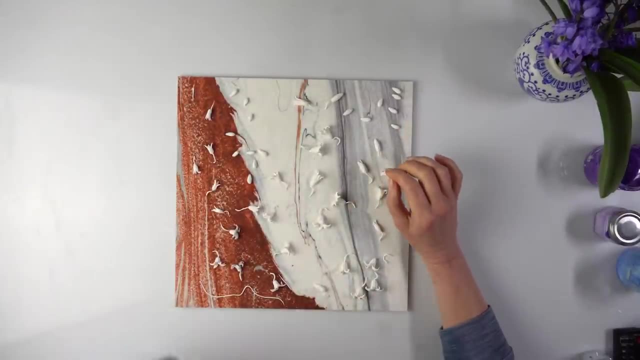 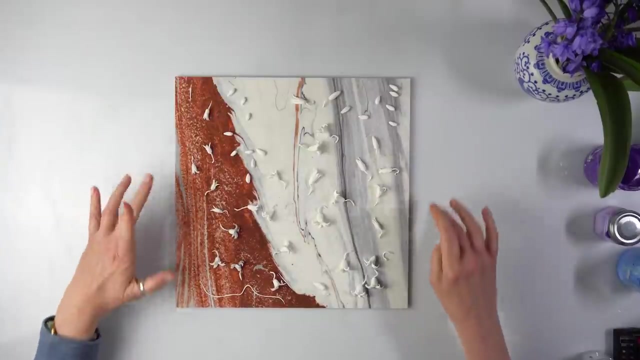 really hard, even those flimsy endings. look at this. uh, all right. so now I'm thinking, if I paint them with a brush, I might paint them with a brush, but since we do have pouring paint, I'll try to dip them in my pouring paint first, see what happens and if I'm not too happy on the the effect, I can. 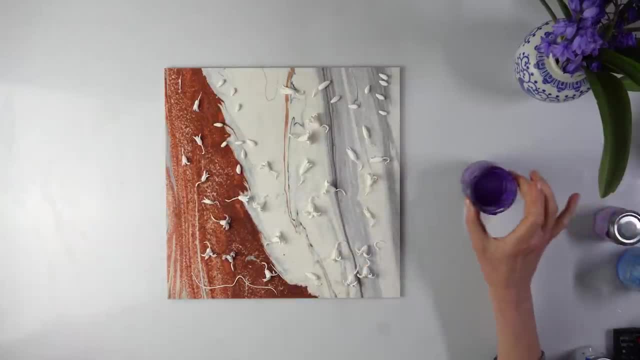 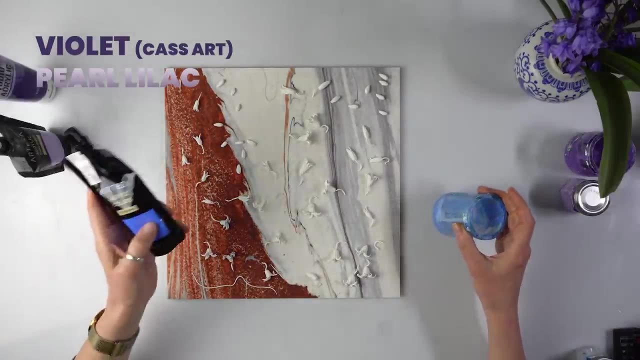 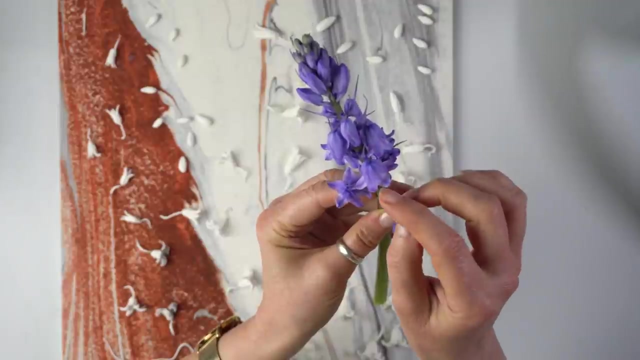 touch up with a brush. So what do we have? I've got some violet by Cassart that I premixed. I do have pearl lilac and I do have leftover cobalt blue. So, looking at those flowers and I'm really analysing the colour now, Yes, you can see the lilac, you can see the purple, but you can see. 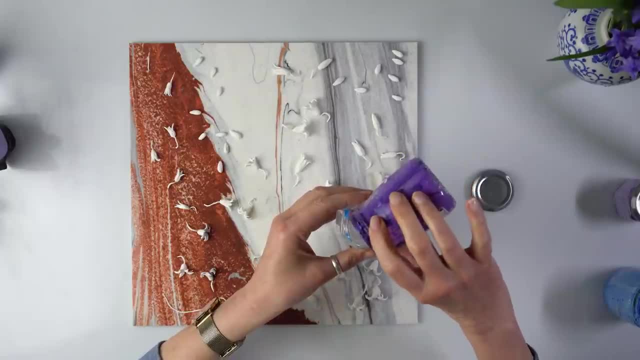 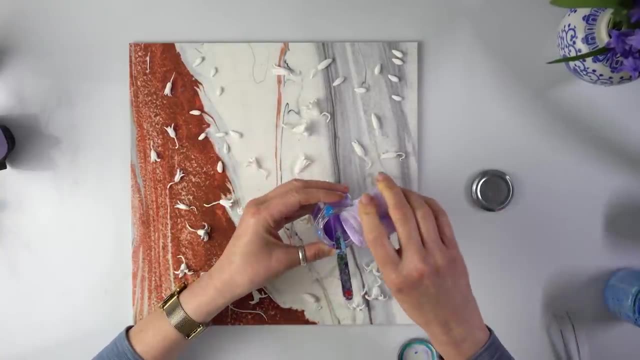 the blue, I think I need to mix three of them. Purple lilac: I'm just going to create a little buff. Well, this is not bad, And a little bit more. a little bit blue. Not much, just a drop. 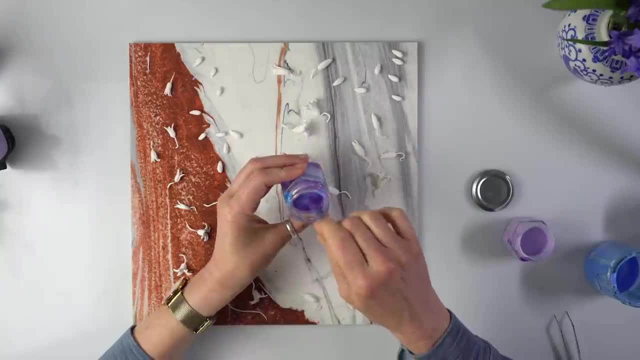 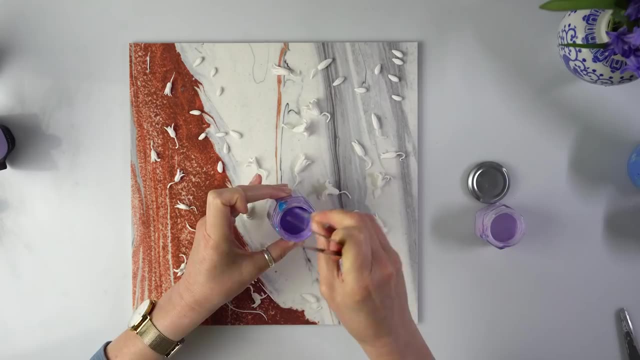 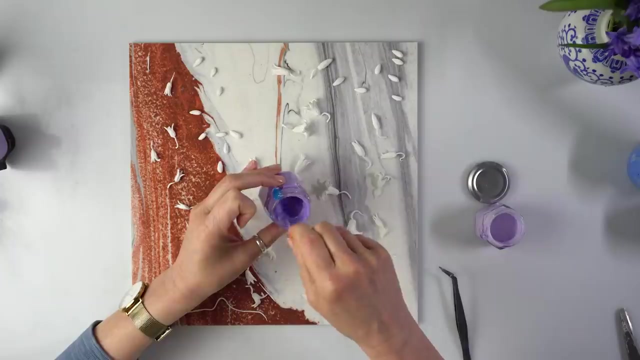 As you can see, this paint is thicker than my average paint and I'm just going to water it down. So what do we have now? Now we have this. I just watered it down. It's pretty runny. It's more runny than my normal mix, but we did have the same ingredients, So there was one part. 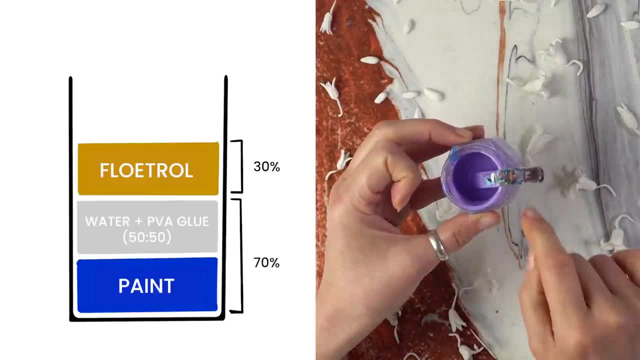 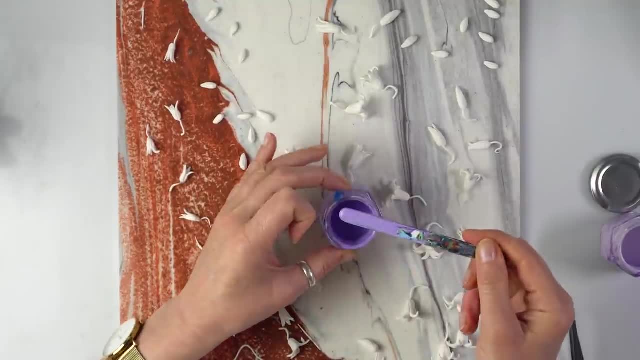 of paint to one part of pouring milk. So I'm just going to add a little bit more of that Medium and one part of flocho, But then I added quite a lot of water. Let's just run smoothly. Why? Because I don't want to clog any of those tiny elements, I just 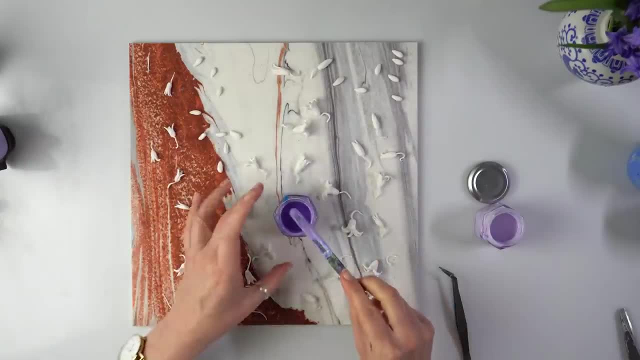 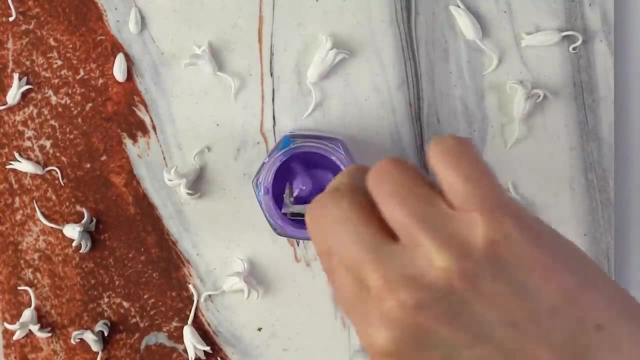 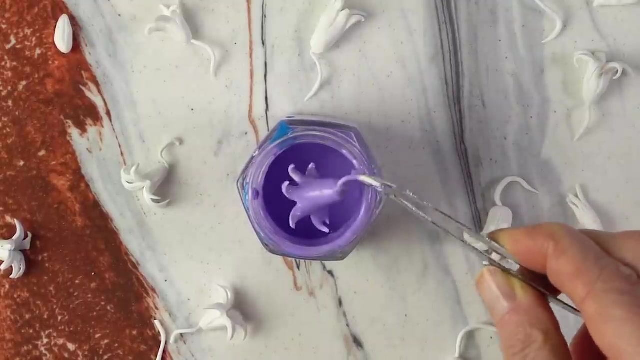 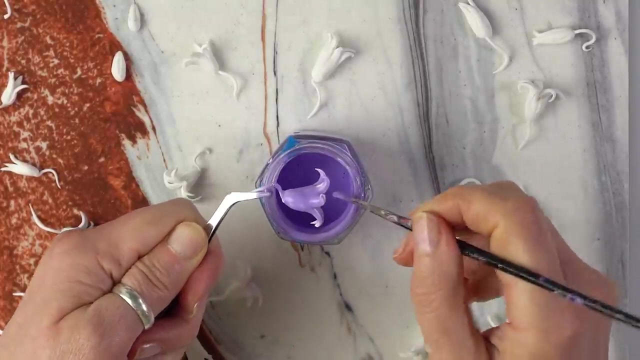 want the paint to drip off the flowers. Perhaps it will drip too much. We'll see, Because if it works, it's going to be the quickest painting ever. Okay, it's not bad. There's some paint here Trapped. I definitely don't want it. 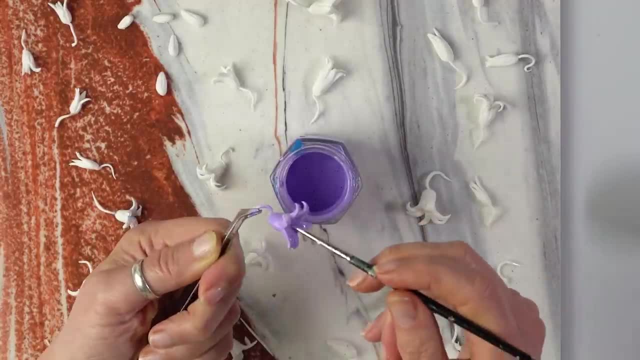 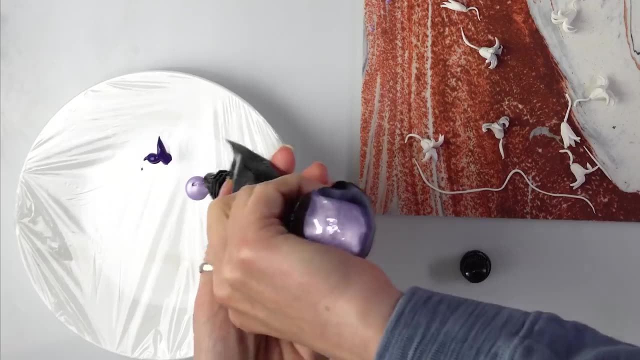 Now I'll see the difference when I paint one and see which one I prefer. So I'll put this away to dry and then see the difference. A little bit of this purple. I'm showing you what to do if you don't have some proper wooden board where you've. 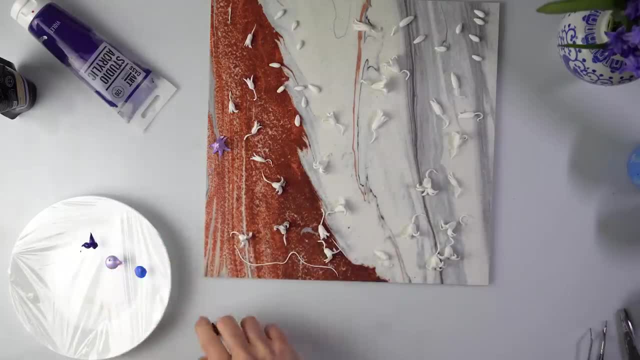 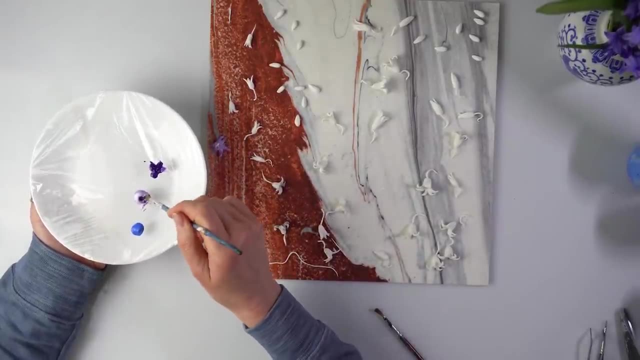 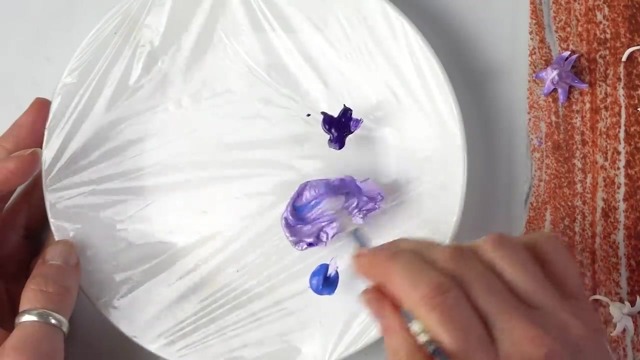 spread your colors. Tiny bit of blue, As I always tell my students. don't ever mix in the darker color, That might be too late. If you do it in the lighter, you can always add more. I'm going to add a bit of titanium white, because this is too shiny for my liking. 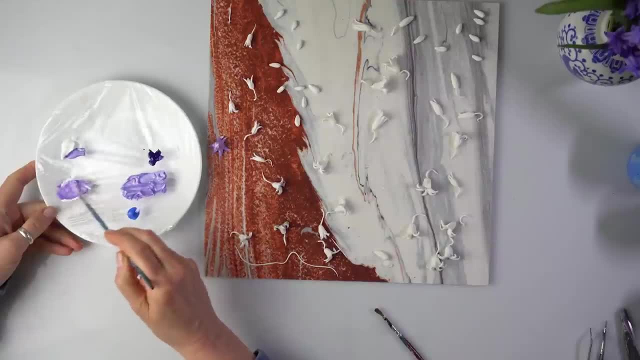 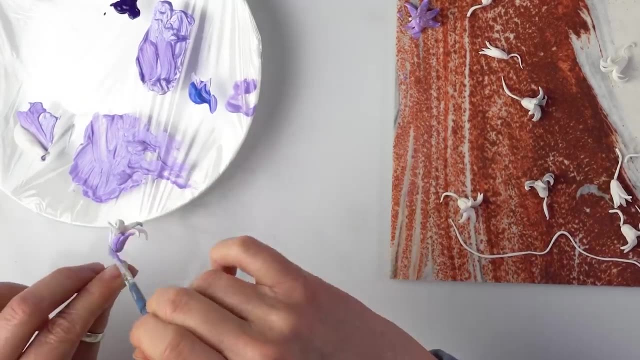 for this particular type of flower. So, as you can see, I added titanium white. I'm ready to paint. Oh, you know what? I thought it would be hard, but it's supposed to be easy. I might do it this way. So that's the one that was dipped. 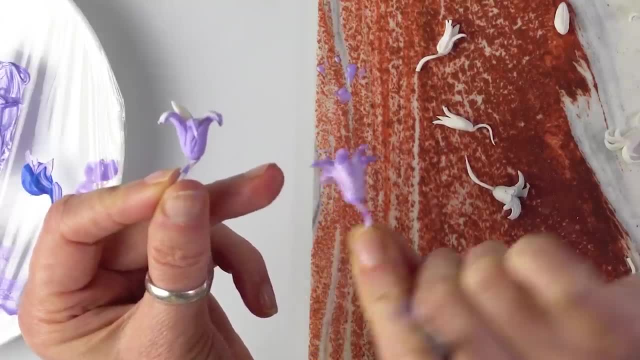 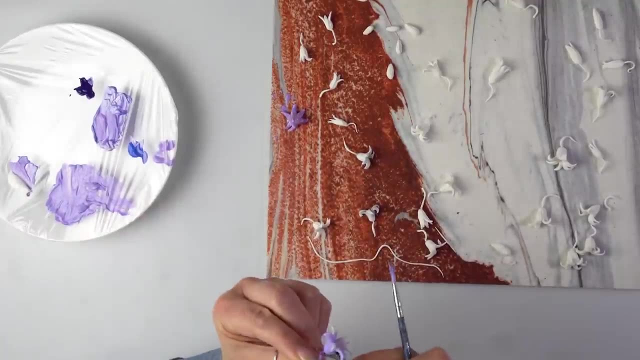 It's nice, but you can see the end's a bit darker. Actually it's not a bad option, So I'm just going to cover those quickly. Again, very therapeutic If you like- and I assume you like, you know, since you're watching my channel, you must love. 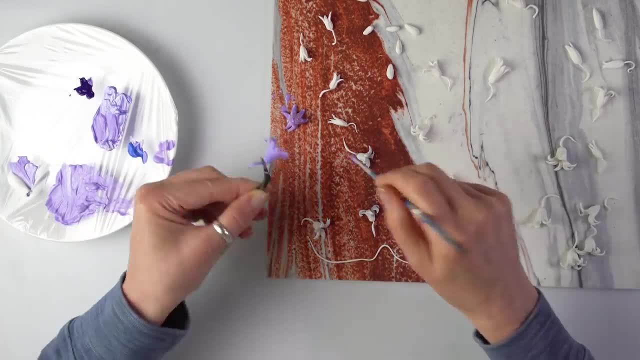 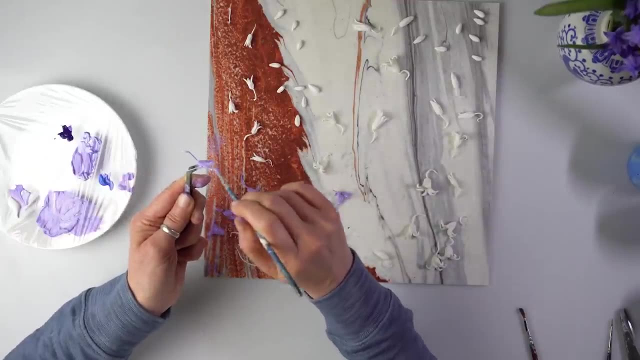 doing arty things, So very relaxing, All right, Very happy with this While I'm painting. I just wanted to mention that, of course, most of you know that you can buy clay in the right color, so I don't have to be painting. 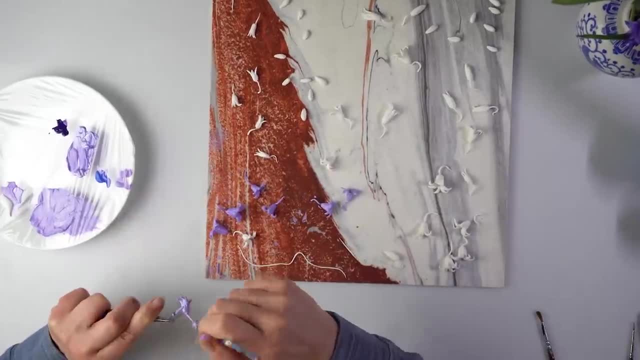 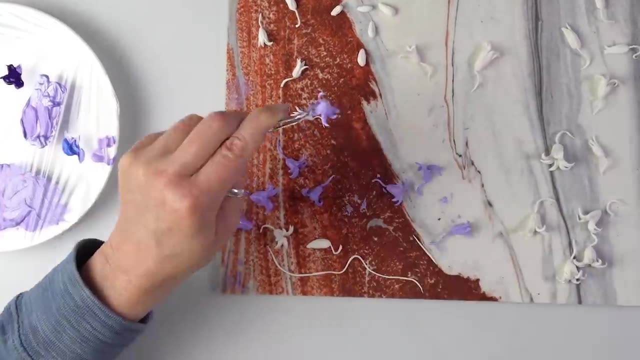 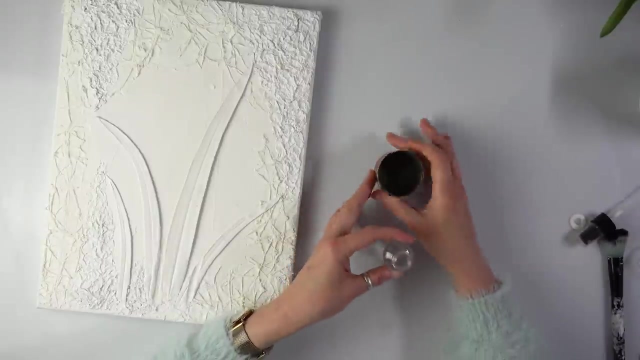 I could just order lilac polymer clay. They've got all the colors possible. You can also add pigments to your Fimo. Fimo is something that I'm still learning. I'm just checking if all the edges are nicely covered with titanium white. Yes, I've got this leftover. dark green, that was. 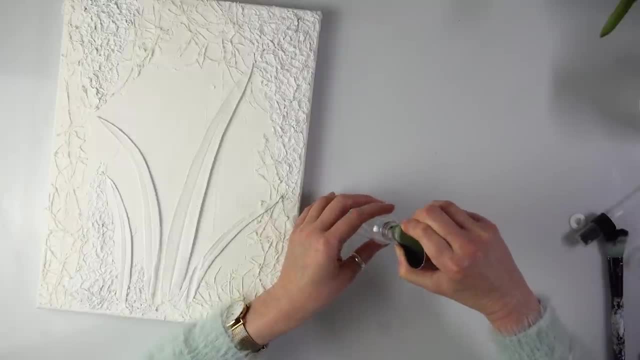 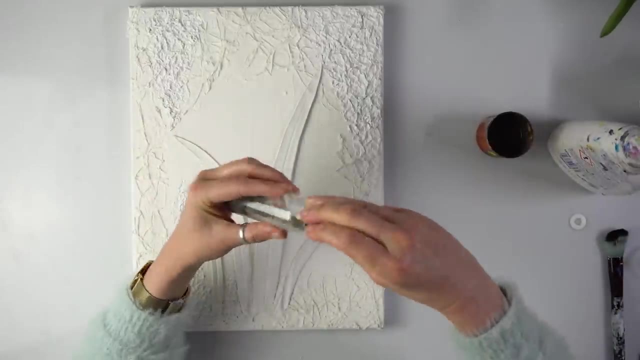 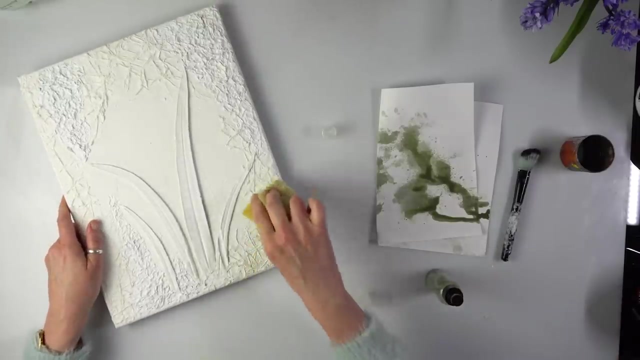 left from my Queen Anne's lacing tutorial- if you watched this one- But I thought if I put it in a spray bottle and heavily dilute it, that might work. Let's see, I'm spraying my paint now. There's a glob, but we can always dab it with a sponge. 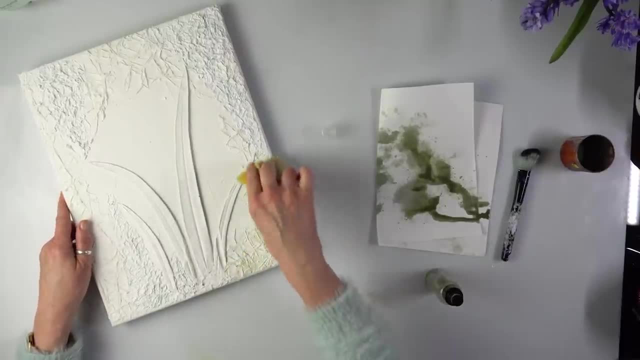 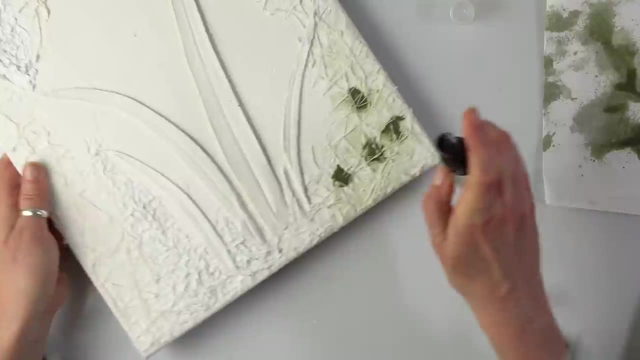 Just make it much lighter, And then I can come back to it later. Let's spray some more. I do want the dark paint to just get underneath into all the crevices. I'm just touching it gently, helping it move underneath. 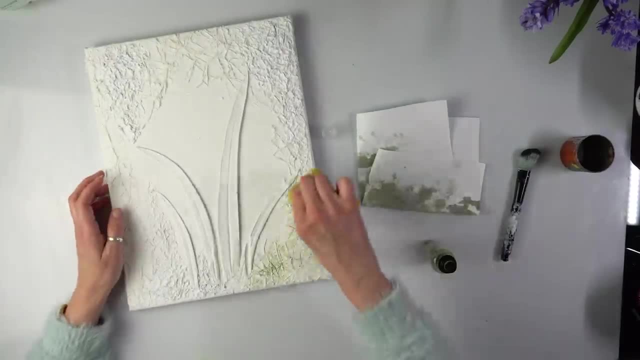 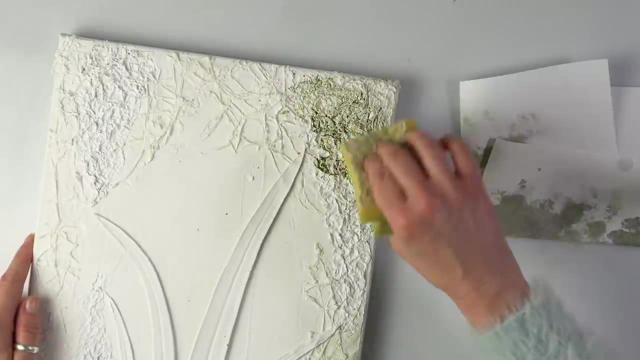 Dabbing again, And I'm going to repeat it all around now. Let's see how the aluminum foil will react. I think we need more paint Sponge to the rescue. I can dab just even. you know, I don't want the center to be completely. 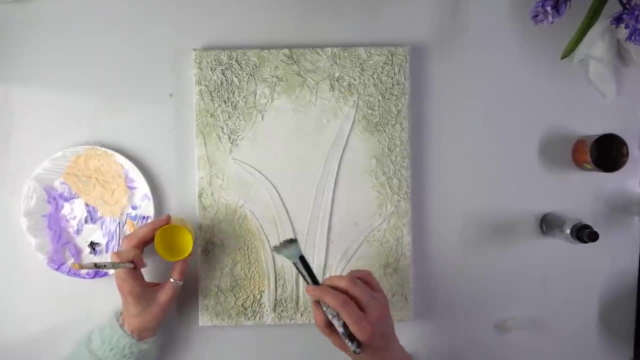 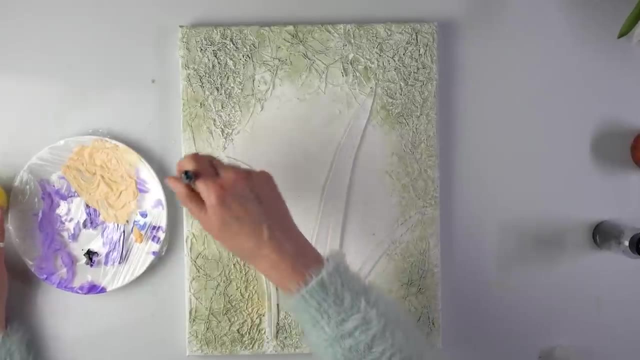 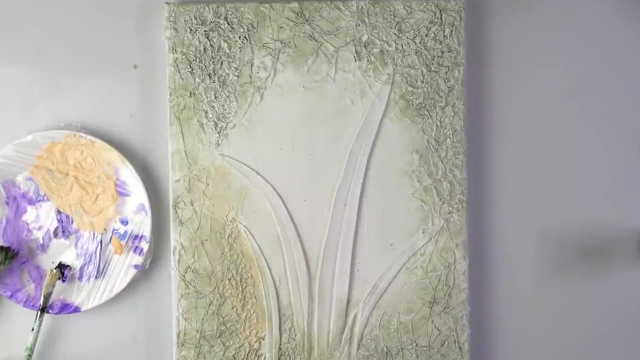 green, but just a little bit, With the edges all camouflaged green. I thought it would be nice to introduce another color, And this is my pouring yellow mix And I added a bit of champagne. I'm using again my makeup brush and dabbing it down ever so softly in between. I thought there. 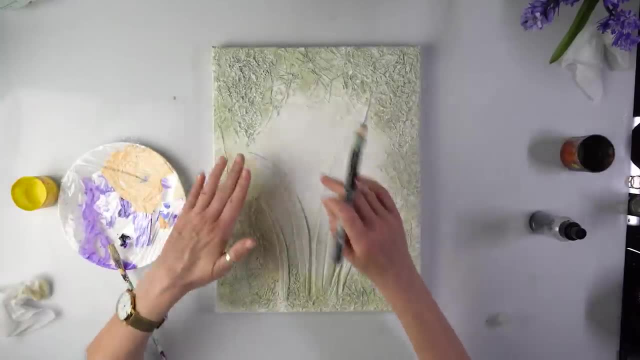 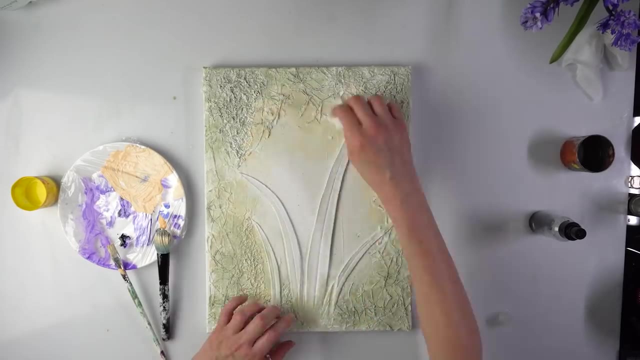 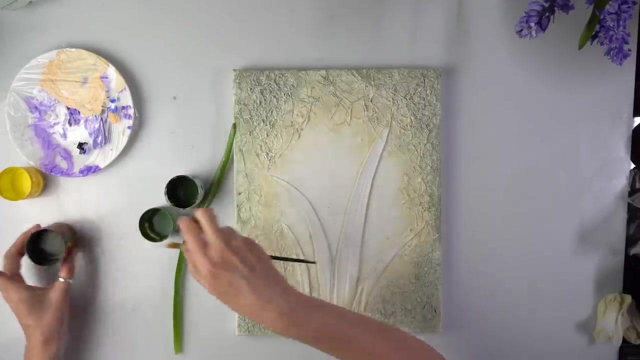 was a bit of a too much of a contrast between the green and white, So I want another soft color just to transition from green to white. I thought it would look nice and soften the edges a bit. Well, time to paint the leaves. I'm looking at the original and there's it's quite a bright green with. 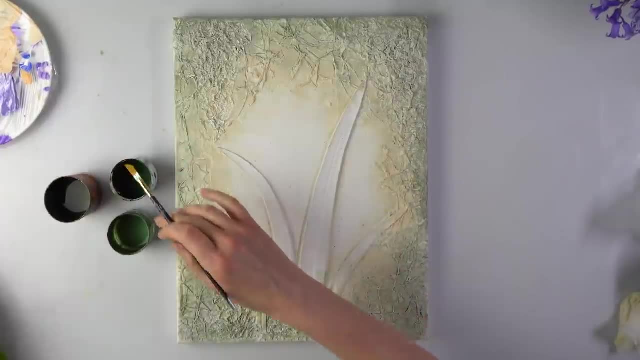 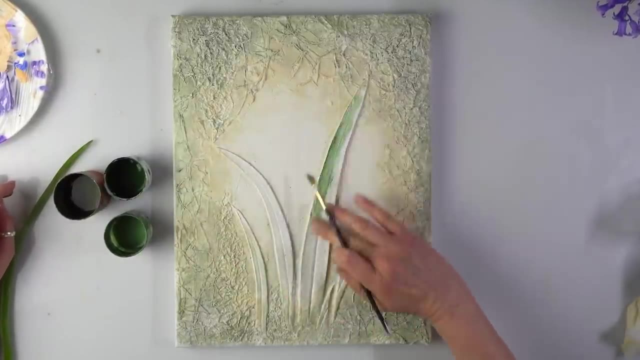 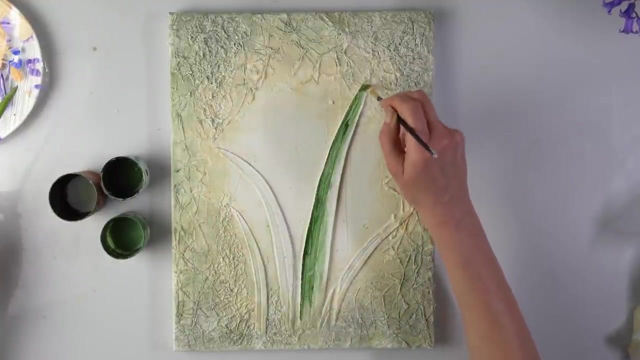 a lot of yellow in it as well. I'll just start with this green first and add one layer Again. I just want a quick wash. I don't want to make it perfect, I want just a hint of green, And then I think I'll come back with another tone, because it's going to be too dark now. I think it's a bit. 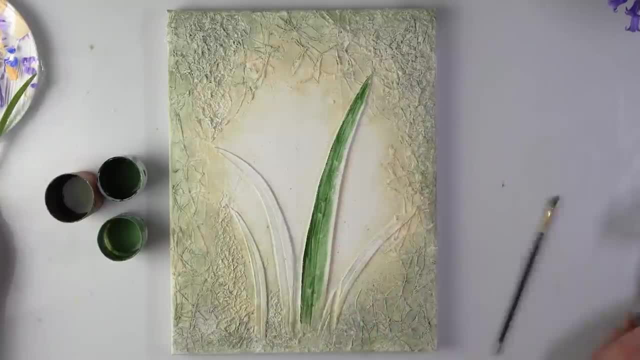 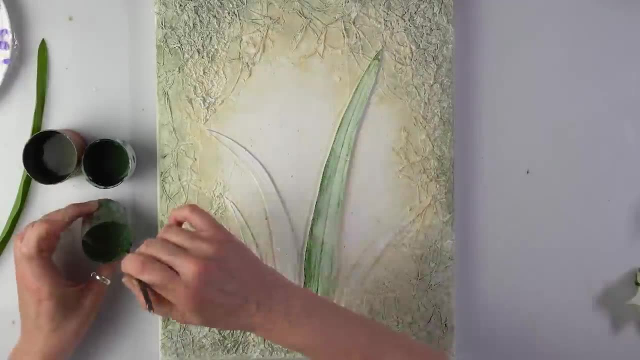 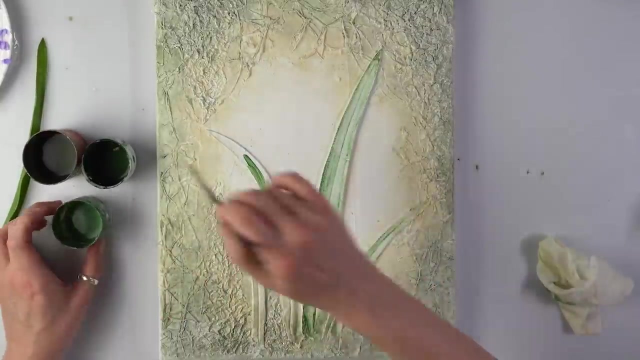 too dark, So I am rubbing most of it off. Well, I think I took most of it off, but I think I'm going to paint all the other leaves the same way And then and then add some yellow, And I think that that will give us the right color. Oops, I definitely don't want any paint. 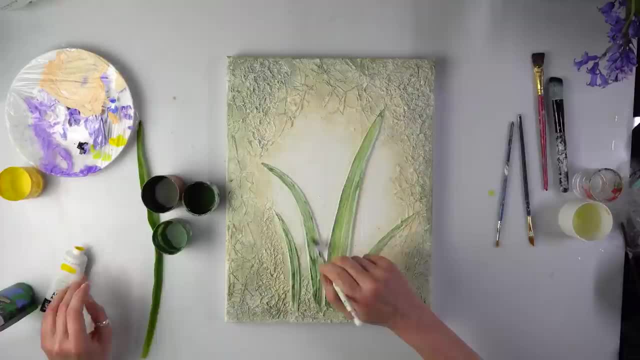 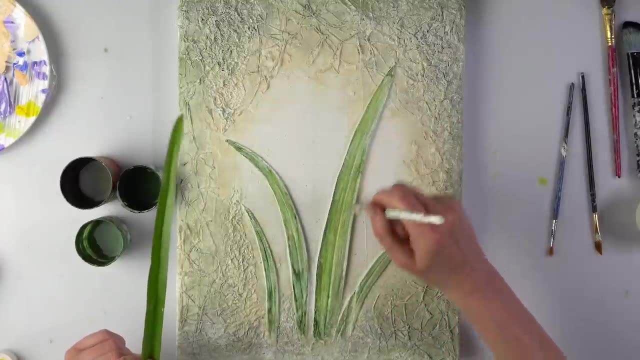 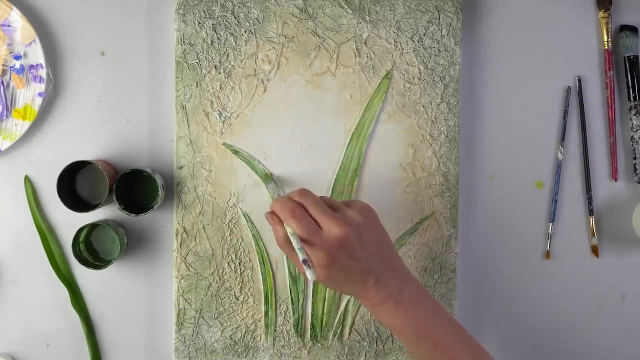 underneath my leaf. I just want the green to be on top. I've got this cadmium yellow And I think adding a bit of cadmium yellow onto this green will give us the right effect. Do you think? Again, not much. As I said before, I don't want the leaves to be really vibrant. 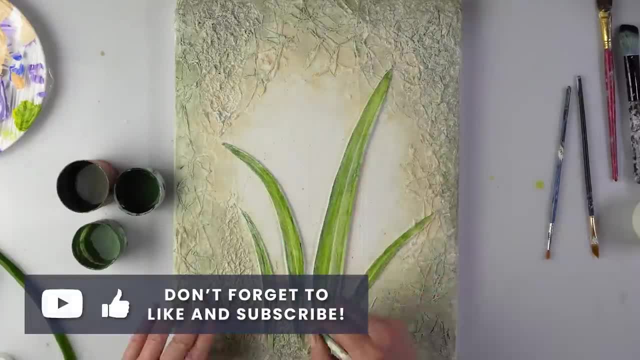 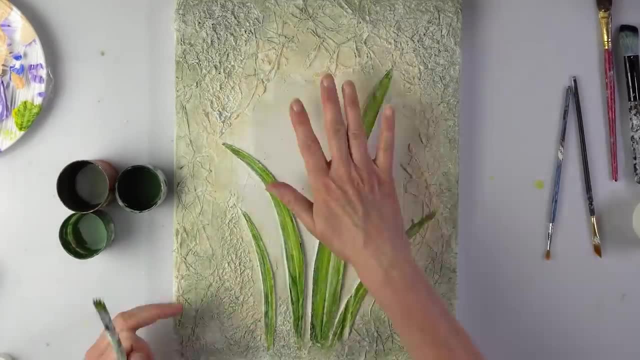 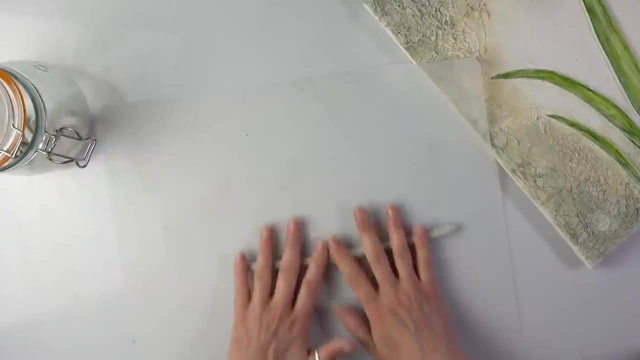 The flowers are going to be the main, the main attraction here And now. I think the yellow goes pretty nice with the cream color we used before in the background Time to roll the stems. now I'm rolling, rolling. It's important to keep the right shape. I don't want it thick in the middle. 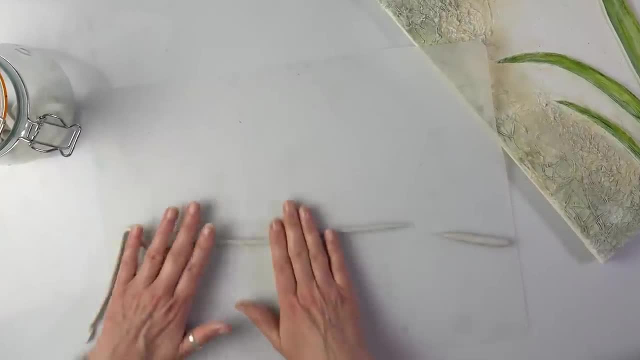 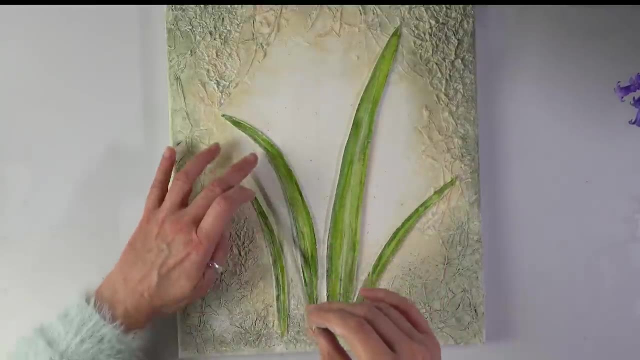 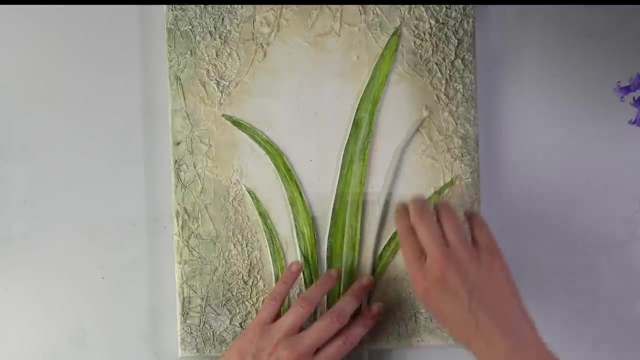 I want it really nicely, starting from thick and then going thinner and thinner. That's a bit too much. I don't think I'm getting there. I think it's going to look better. on the right: Yes, that's the right position. I think A little bit curved. maybe It just fits into that. 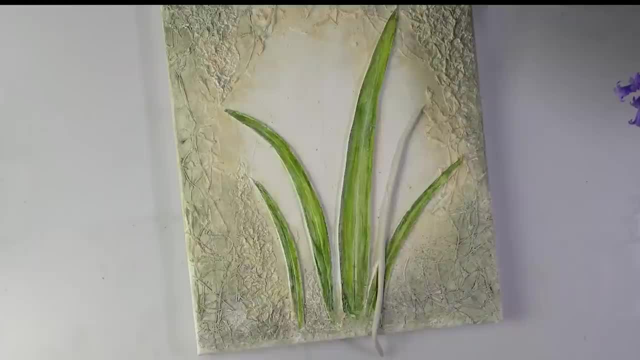 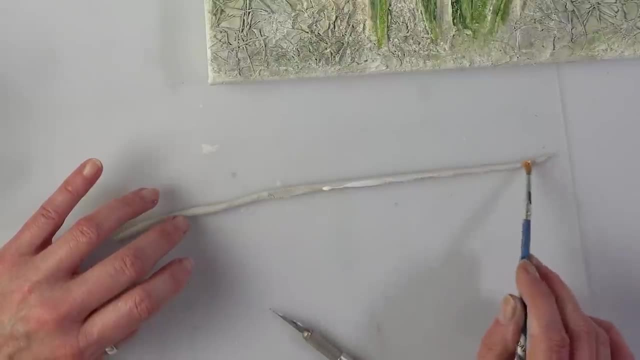 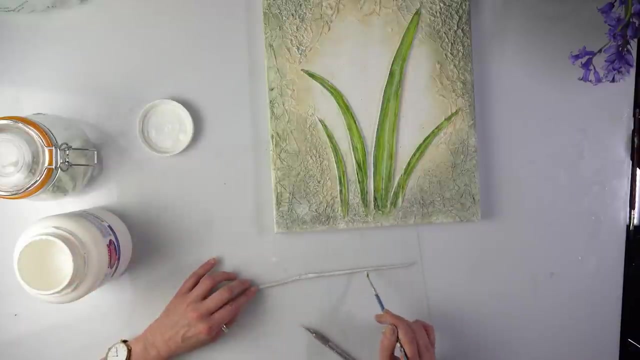 Do you remember that little crevice we made, the little hollow section we made, And I'm using my PVA glue and covering the stem evenly, spreading the glue nicely. Now this is the same PVA that I use for my pouring mixes And there's a link in the description for this product and the American. 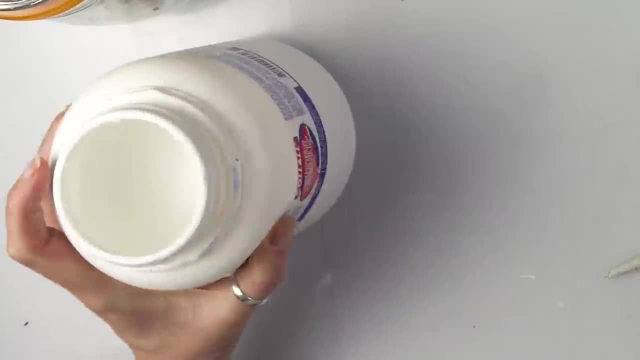 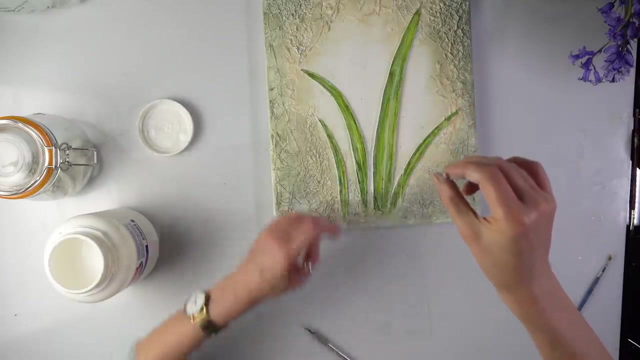 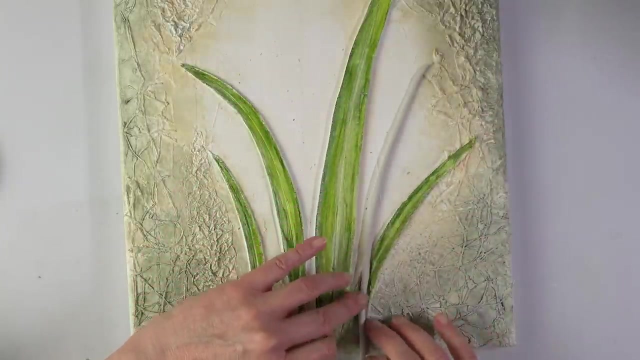 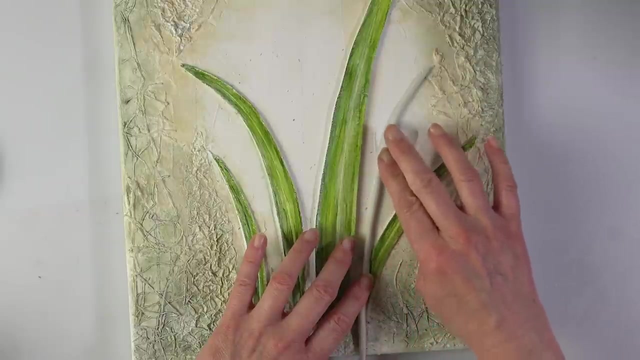 version as well. It's really nice, It's archival, It's very strong, really thick. I really really like it. Now, super careful, Where will it go? I'm going to add a little bit of bend Now, tapping, tapping, Make sure it adheres really well. 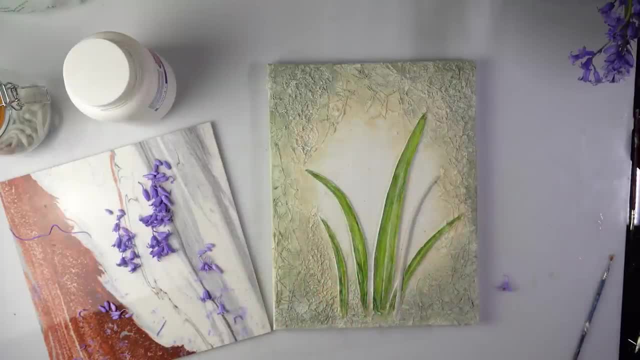 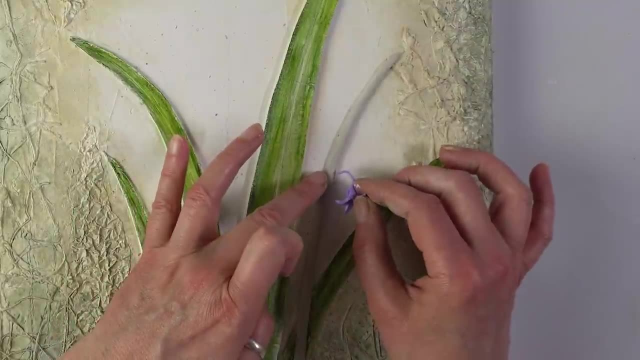 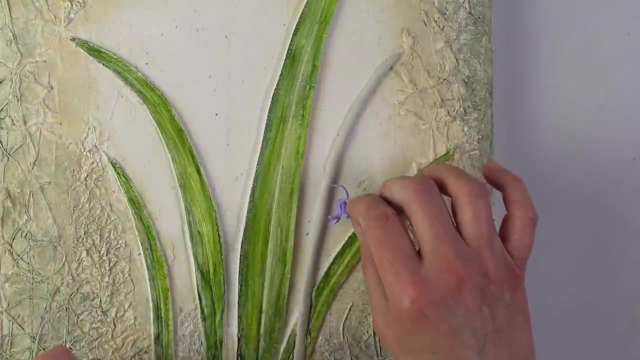 Now I'm going to tell you why I wanted to add the stems at the very end, not together with the leaves, because I wanted them soft. I wanted to be able to poke the stem through and attach my flower. I thought it would hold it really nicely. So that was my thought. So let's try how it works. 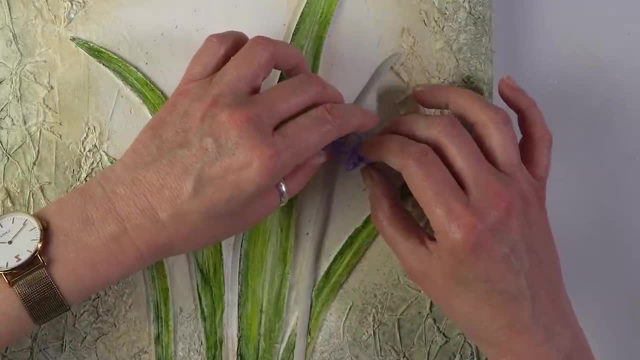 And, yes, I'm going to add a little bend Now, tapping, tapping, Make sure it adheres really well. I'm going to use glue as well. I'm just trying them out first to see which position I want them in. Let's open the glue. 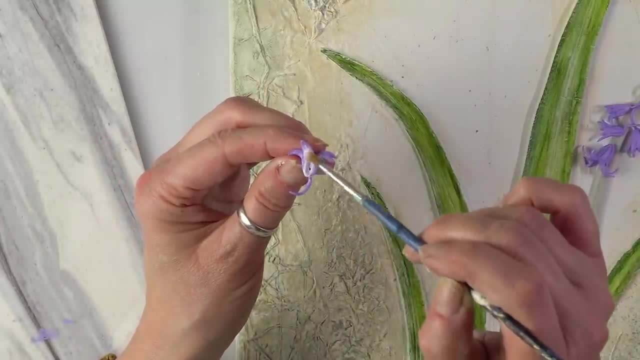 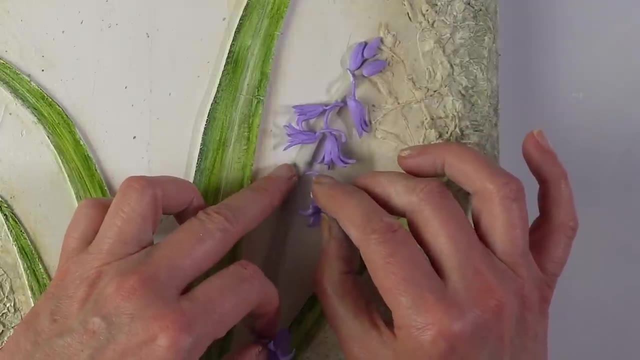 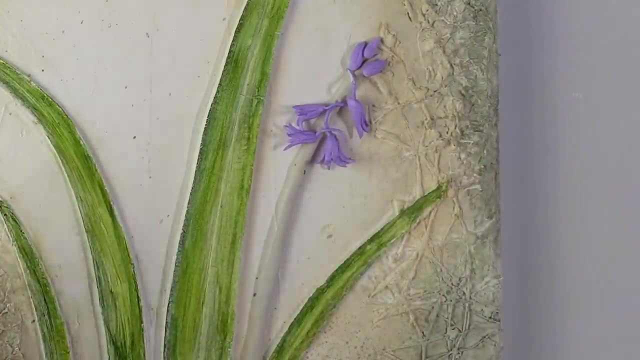 Checking where the bottom part is and just gluing that flat section, And then let's poke it through the stem as well. I think it was a bit too long, so I'm going to snap it. That's better. Okay, first one done. 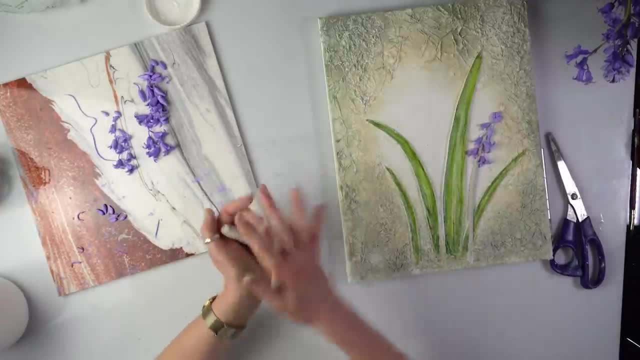 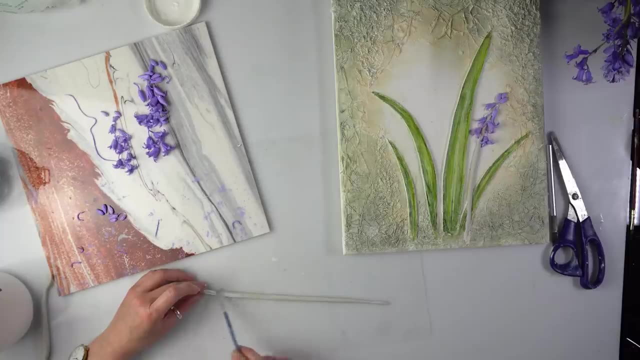 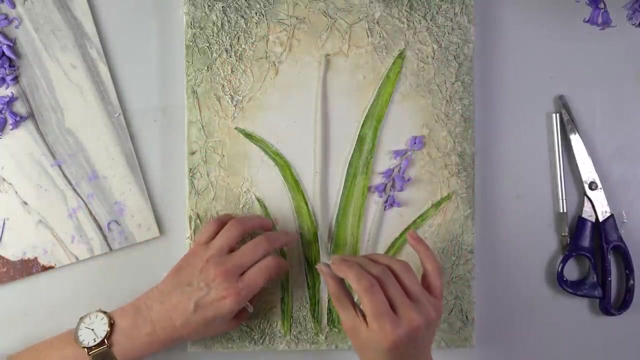 I'm rolling the clay for the chunkiest one. Again, I want it nice and even, Of course, thinner ending, tapered edge Gluing carefully the thick one, Positioning just in between. There's a space in between. I'm going to make sure the end is nicely stuck. And now time for the glue. 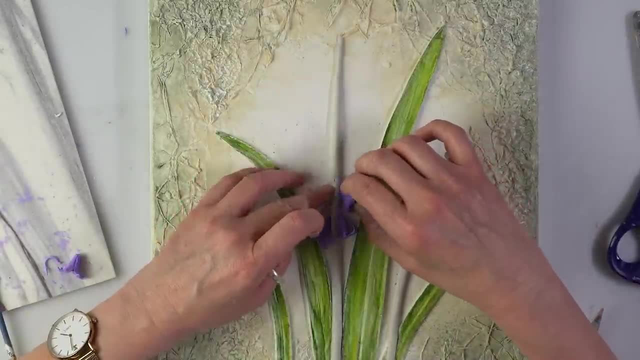 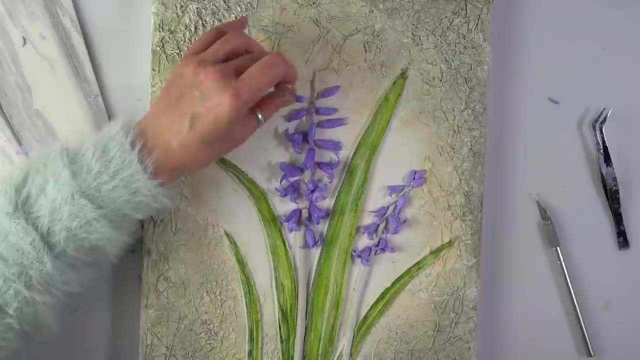 Let's poke it through the stem. This is a chunky stem now, so it will go nice and easy. Now, glue gun is better for the little ones, so I just need to add those few on the top And I think one is going to be slightly overlapping. 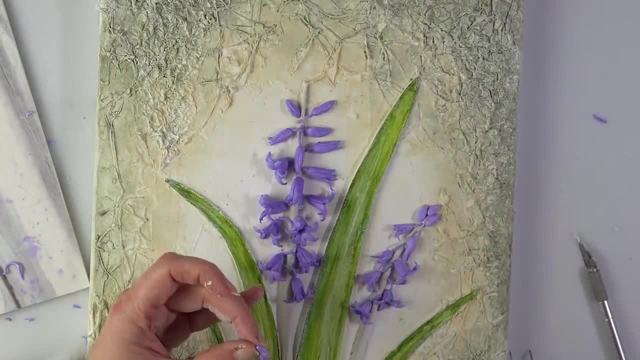 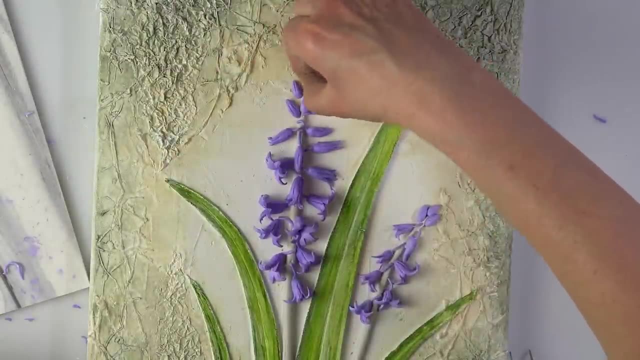 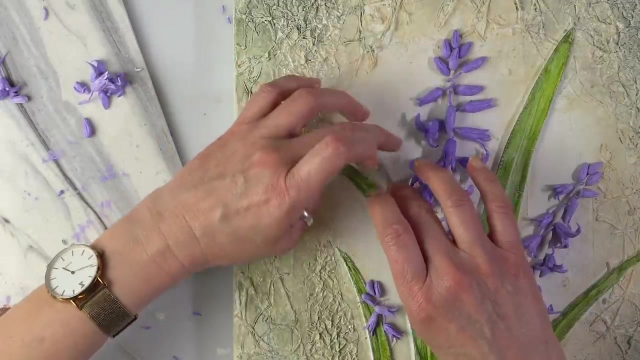 I want this one just in the centre, So I'm putting it directly onto the stem And the very last one on top And we are done. Now. I wanted one of the stems to be partially hidden behind the leaf, so I just have a really tiny bit now. 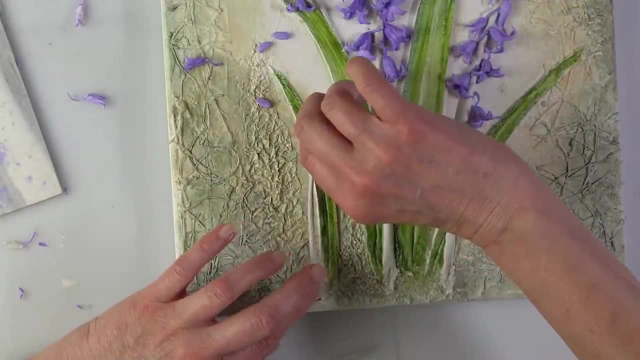 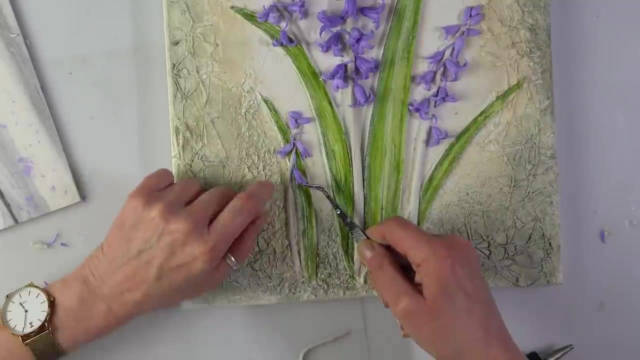 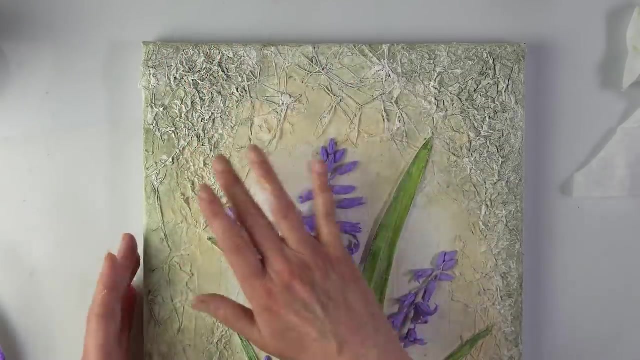 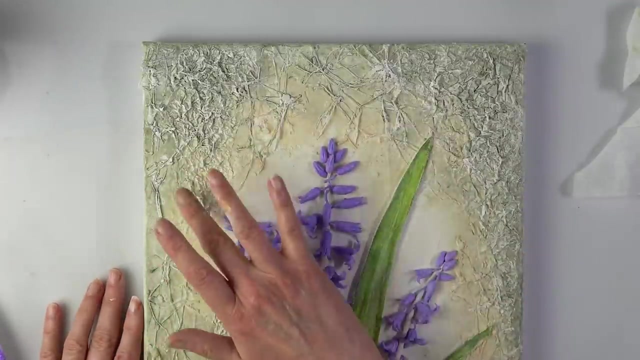 What about overlapping the leaf? That might look good, What do you think? Alright, so now I can start gluing the flowers And pressing it down onto the leaf. I think some of my edges lost a bit of definition, so I'm trying to recover the texture with Titanium White before I'm going to use gold. 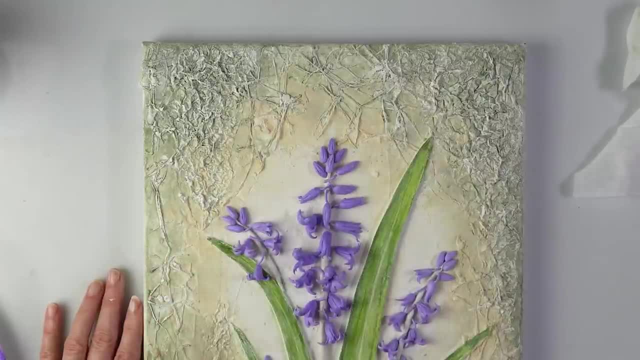 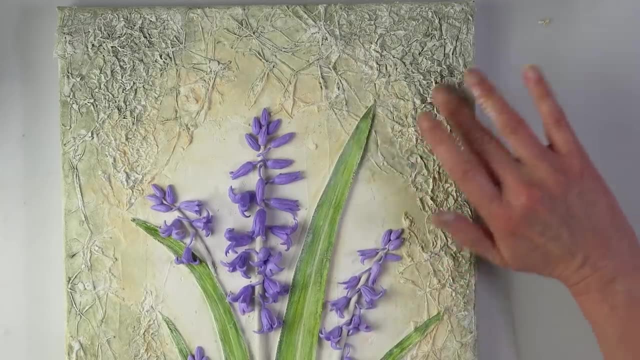 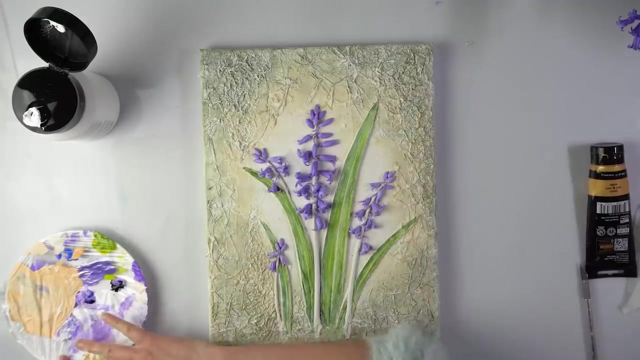 Gently touching with just the very tops And you can see how all those little formations are even more, even better seen. now Time for some glamour, Spark of gold. Can you see the shine? It's like applying Some foundation or some cream, Very gently rubbing. 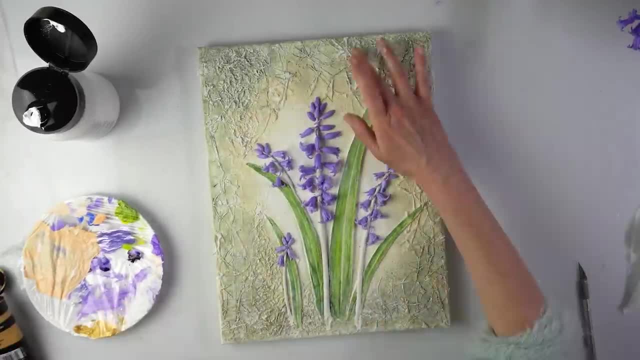 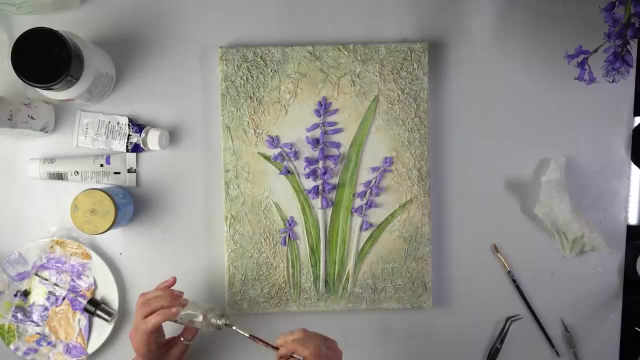 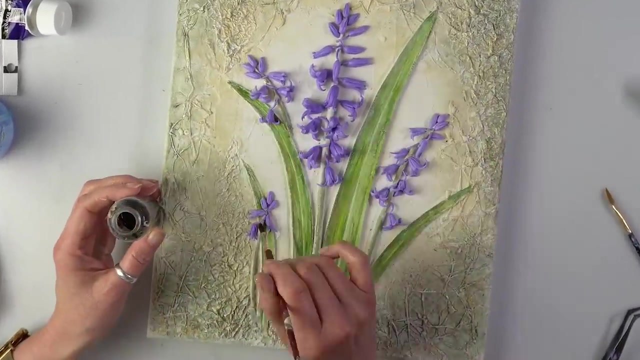 And of course, I'm going around and touching the aluminium foil. I really like the effect. I think I'm going to use the aluminium foil more. The stems are still quite wet, but I thought I'm going to try and just touch touch them with my diluted green colour. 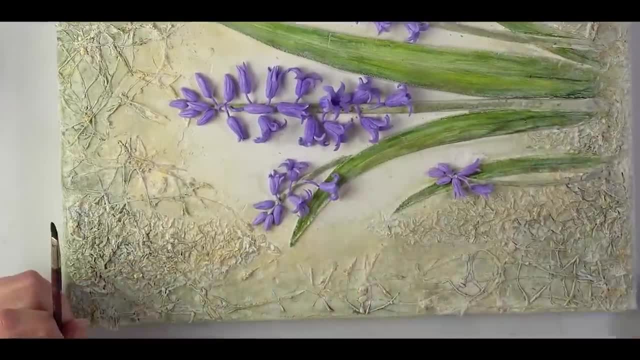 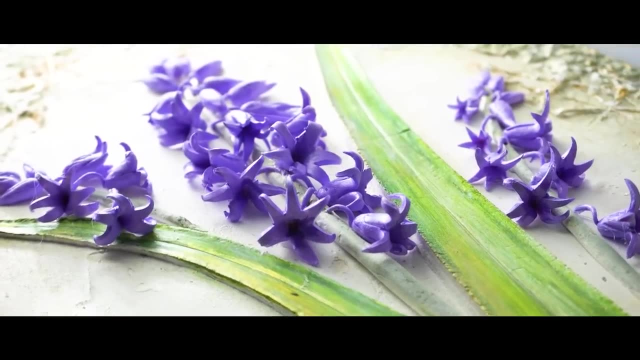 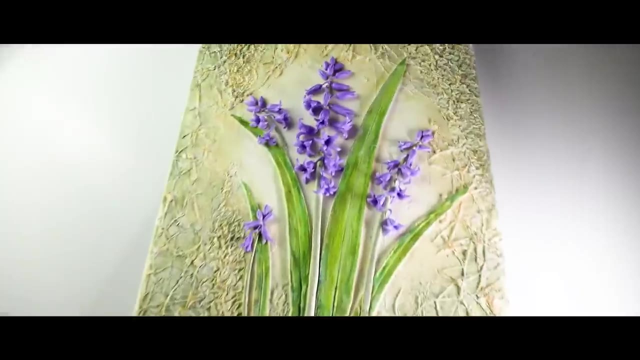 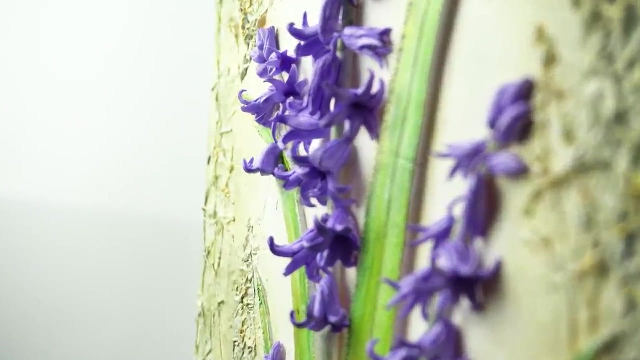 And it's actually because there's so much water it looks like it's sinking into it. Well, all ready now? Well, there we are. I'm going to be honest, this was one of the most difficult videos ever for me to make, And my son was really sick the entire time editing.